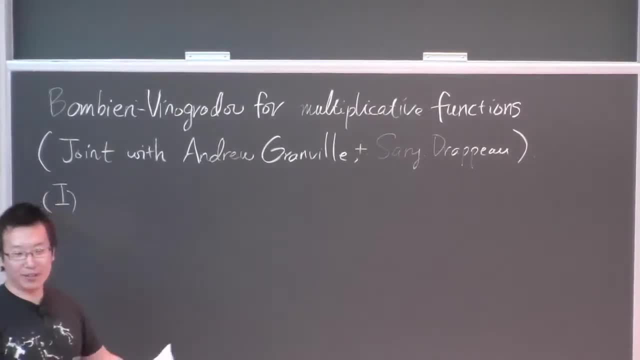 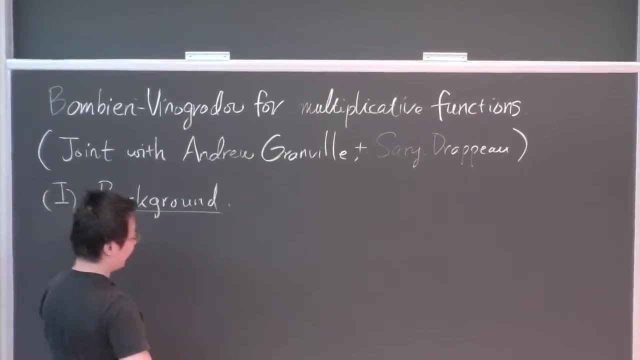 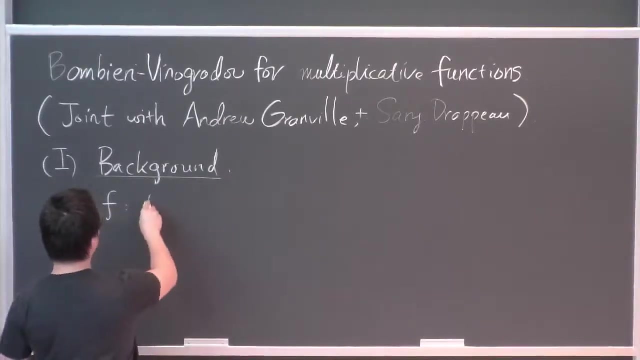 I'll tell you what the Bombay-River-Vinaigrette theorem is and then pose the main question that I want to consider in this talk. So let f be an arithmetic function. By that I just mean a function from the positive integers to the complex numbers. 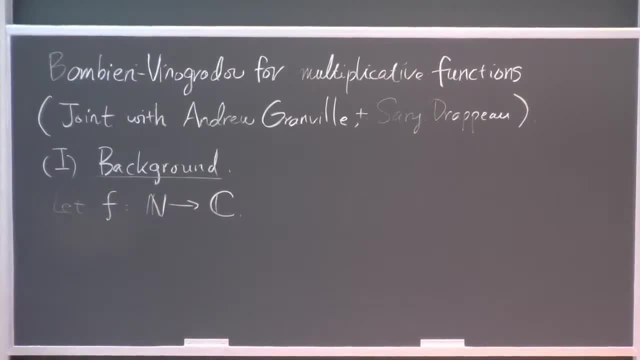 For example, the interesting arithmetic functions will be the von Mangold function that captures primes, or things like Mobius functions, smooth numbers and so on. So an important question in analytic number theory is to understand the distribution of these functions in arithmetic progressions. 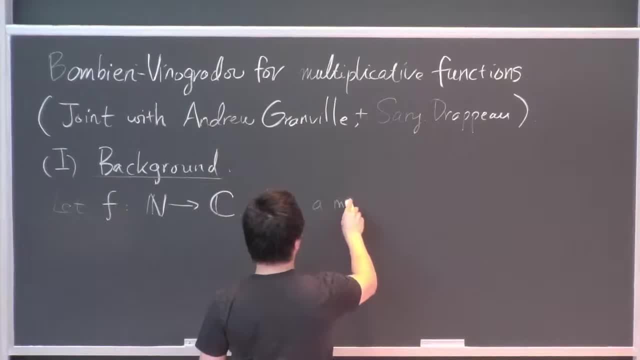 So for a reduced residual class, a mod q, that's 2.. So, for example, if we define the quantity Delta, f, x, a, q- just to be consistent with my note, qa, Ym, Ym, ym, Ym. So if let yk times t is less than 0. 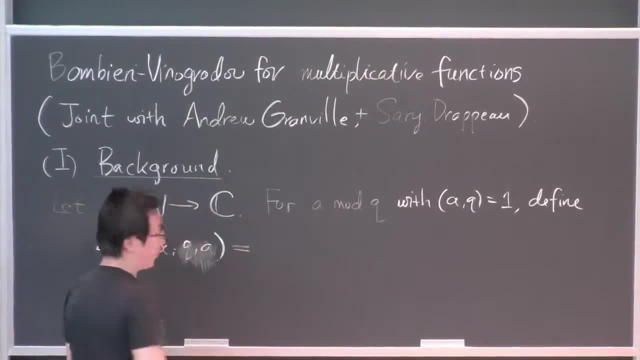 This measures Um well equidistributed. the function is in the residual class A mod Q. So sum over N up to X in A mod Q, minus the expected value 1 over phi of Q. sum over all N up to X, co-prime. 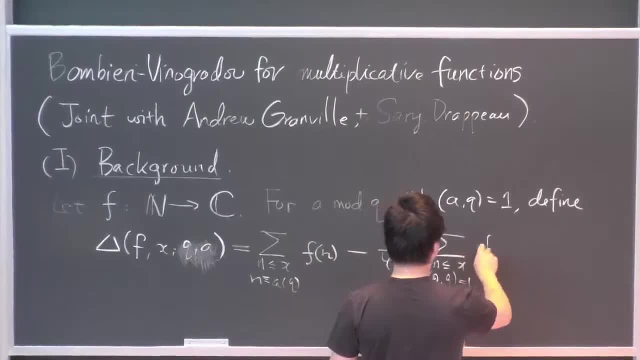 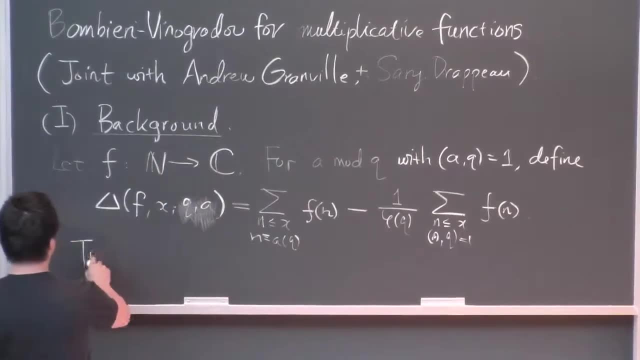 with Q. So note that this has a trivial bound, which is X over phi of Q, assuming that the function is one-bounded. So for most nice functions, F, we would like to understand to what extent can we improve on this trivial bound? So, if we can improve on this trivial 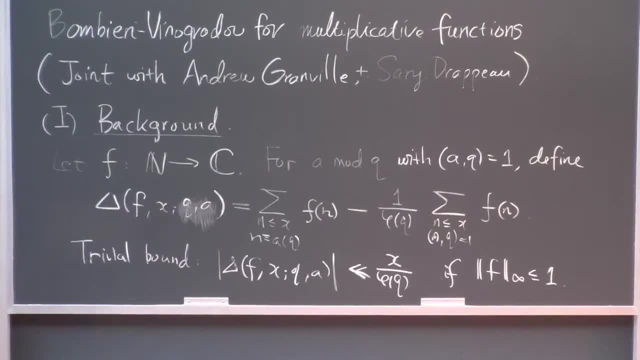 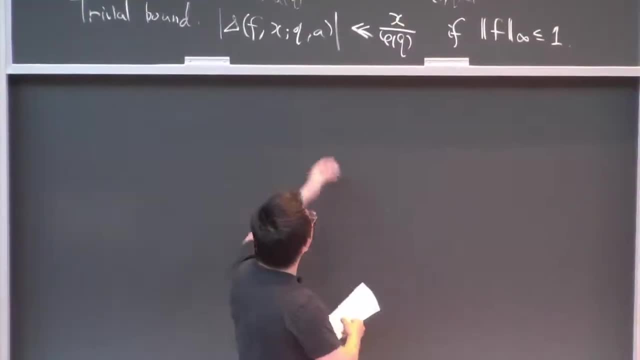 bound, then we may believe that the function is well equidistributed in progressions. mod Q: OK. So in the case of the Vomengold function we have the following theorems. First of all we have the Siegel-Wolfish theorem that says that the Vomengold function is well equidistributed. 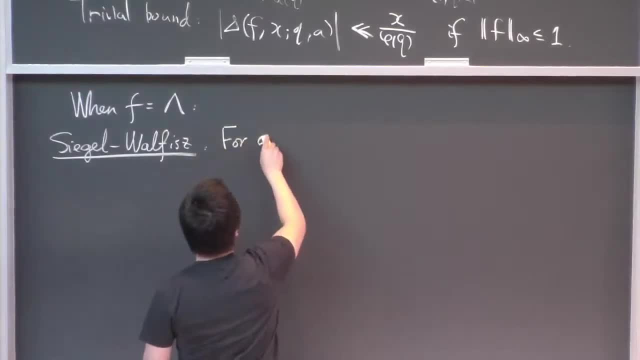 in small moduli. So for any A- Q co-prime, we have the bound, which is X over log X to any fixed power A. In words it says that primes are A Q co-prime. we have the bound, which is X over log X to any fixed power A. In words it says that primes are 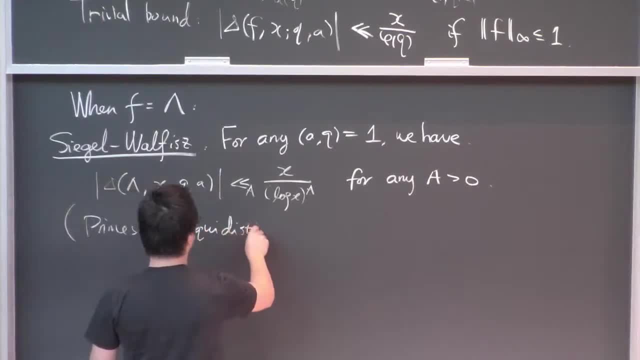 is equal equidistributed mod Q for all Q up to a fixed power of log, Chronically probably even more. This is what is best known unconditionally but conjecturally. we should expect equidistribution for a much wider range of Q. Second of all, we have the 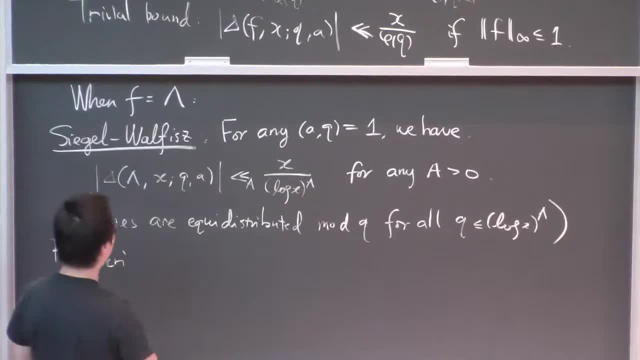 Second of all, we have the second and fourth 치배�ytt out of theorem, which will be the main topic of this talk, which says that if you only want this information on average over Q, then you can do much better. For any A, there exists a constant B depending on A, such that if I sum, or equivalently average, 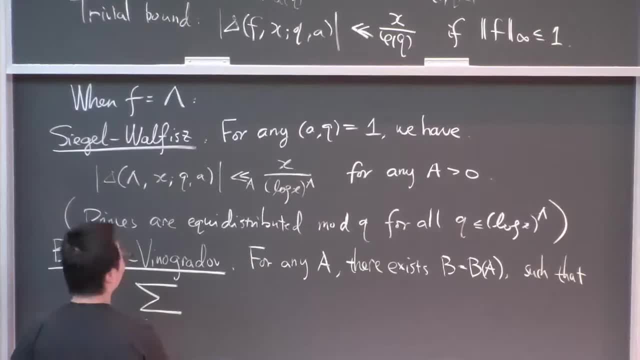 over all primes, sorry, over all Q up to x to 1 half, over log x to B. And I look at this, This measurement of equidistribution. Then I can get log x to the A, saving compared to the trivial bound for any A. 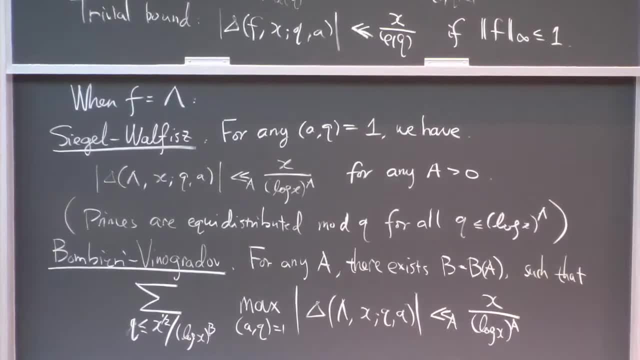 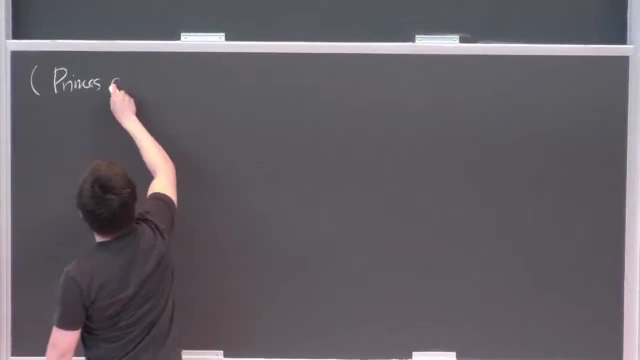 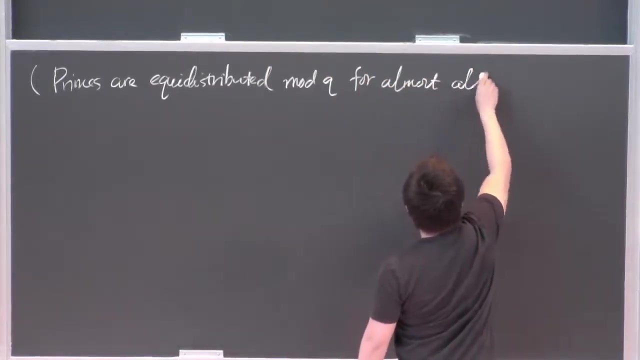 So in English words this is saying that primes are equidistributed, mod Q for almost all Q up to roughly x to 1 half. OK, so, assuming GRH, we know that the Ziegler-Wolfe theorem or the equidistribution of primes are. 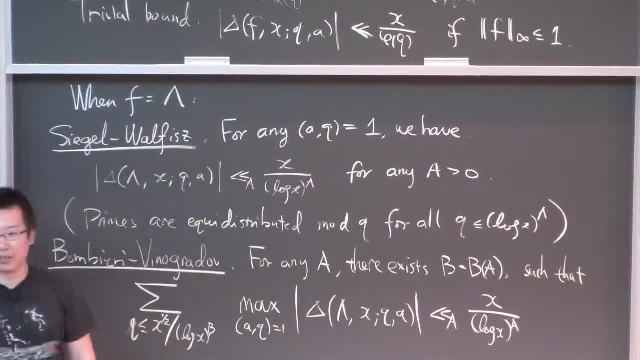 true for individual Qs up to x to 1 half minus delta, And for this reason the Bonbier-Rivina-Gradwitz theorem is sometimes referred to as the GRH on average, At least as far as the application to prime, the arithmetic progressions are concerned. 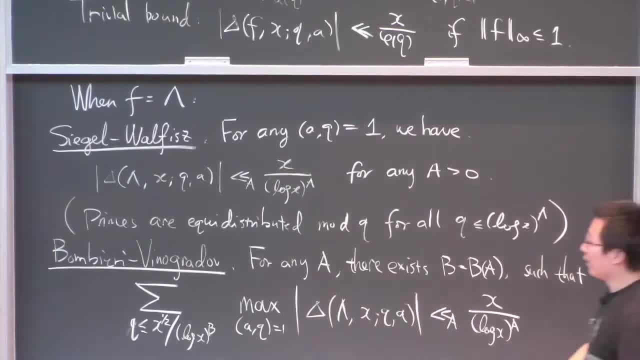 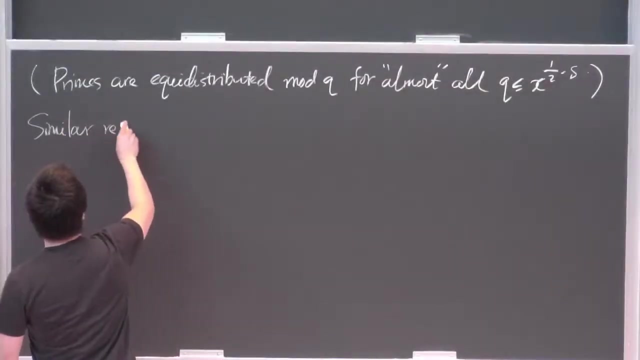 And in many other applications it was important to improve on this level of distribution- x to 1 half- But in this case, in general, this is the best level of distribution we currently know. OK, and there are similar results for other arithmetic functions such as the Mobius function. 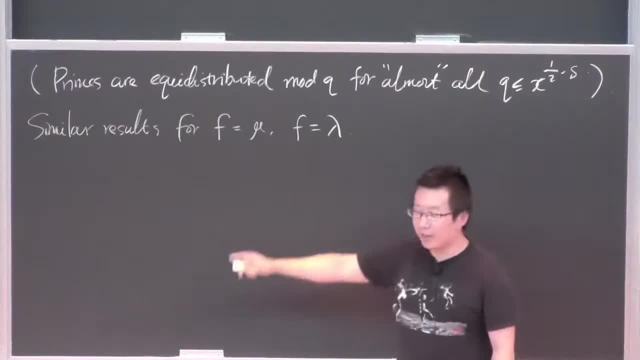 or the Louisville function. The proof for these go along the same lines as the proof of the Bonbier-Rivina-Gradwitz for primes, And also in the case when f is the indicator function of the smooth numbers. So this is: 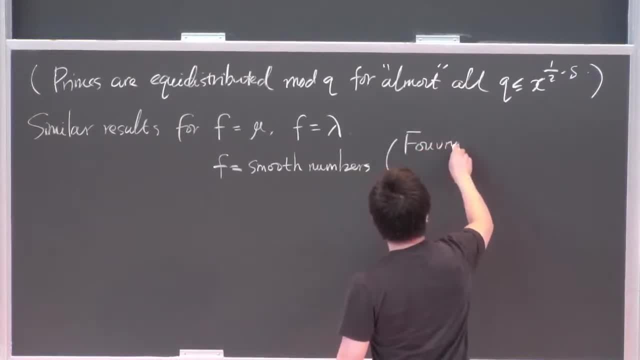 OK, This is a work of Fouvry and Tenenbaum And, for a wider range of the smoothness parameter, a work of Harper. So the goal of this talk is to prove analogs of the Bonbier-Rivina-Gradwitz theorem for 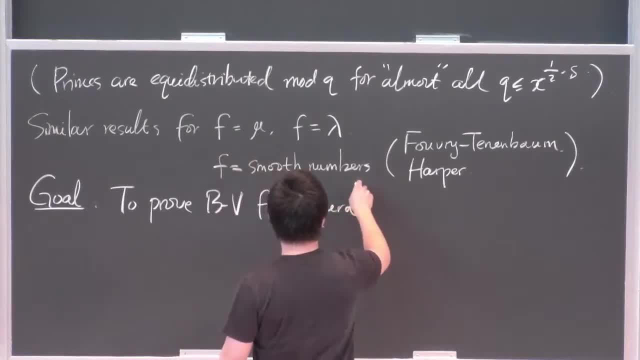 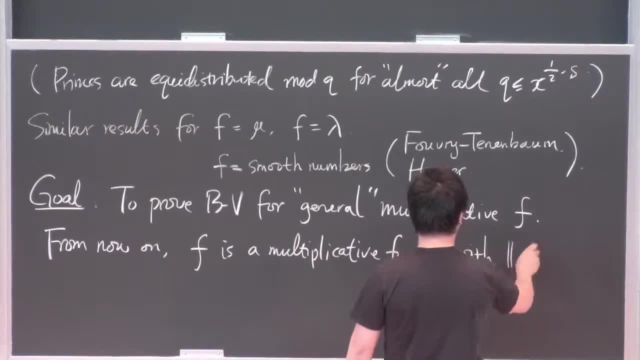 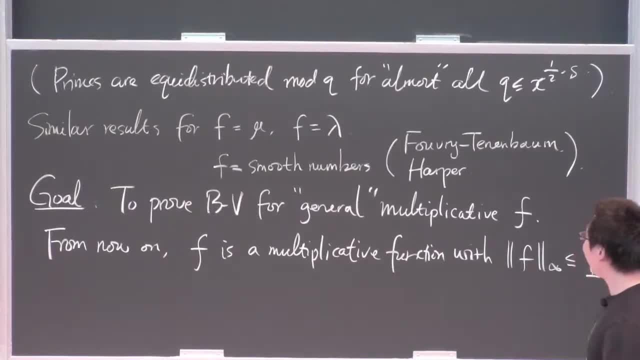 And before I go into any of the details, let me just give you a high-level summary of what is going to happen in the next 15 minutes. So we proved such a theorem, the Bonbier-Rivina-Gradwitz type theorem, for general one bounded multiplicity. 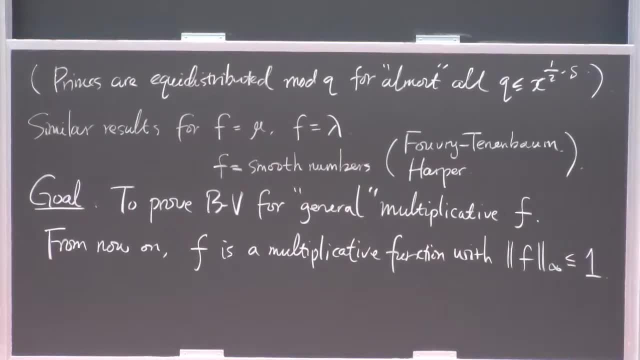 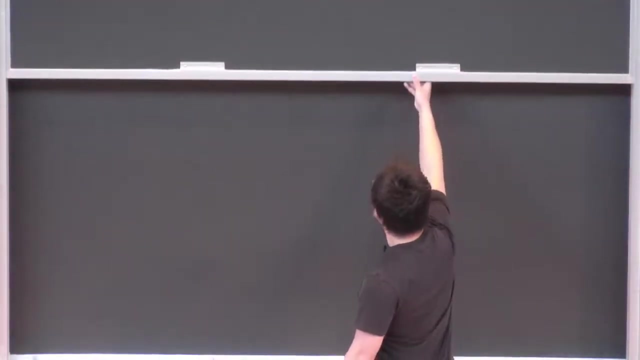 functions. The statement is exactly what you would expect if you're expert in this area. However, we also developed some limitations which may have some novelties and also the proof in our. some of the ingredients in our proof could also be useful elsewhere. 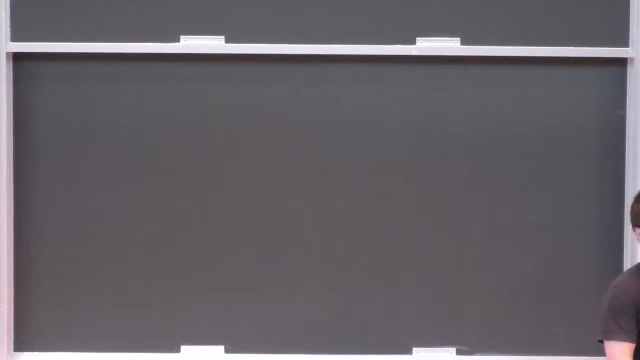 Any questions so far. So before formulating the results, I want to point out two things. First, I said that I will work with general multiplicative function, that's one bounded. It's not quite the case. For technical reasons we study a class of function that is slightly 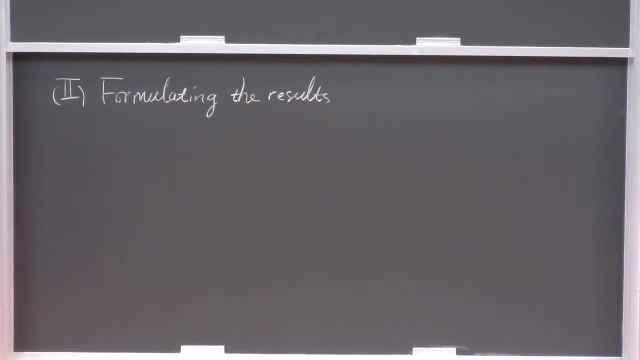 smaller than those functions. I'll, for preciseness, I'll define it, but don't worry too much about that. So let C be the class of all multiplicative functions, because it's not quite the case. So let's start with the first one. 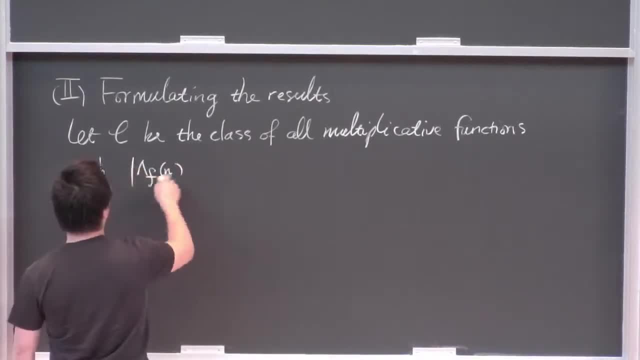 So the first one is the associated function bounded by the actual function. So here, lambda f is defined by the Dirichlet series minus f, prime over f. So I'm going to use this. So I'm going to use this. 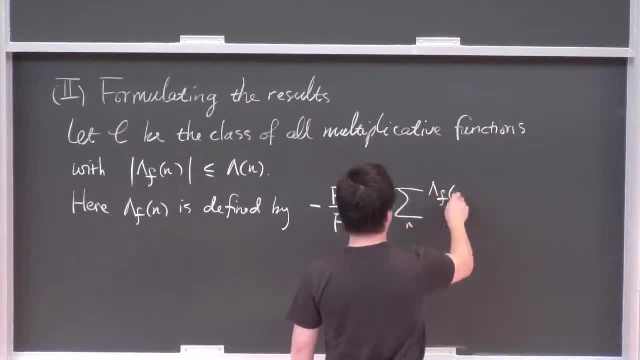 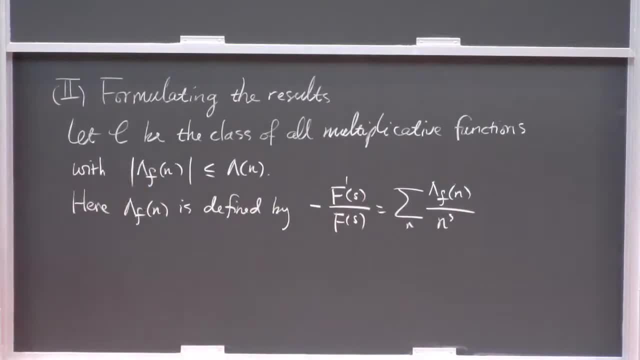 So I'm going to use this. And the capital F is a Dirichlet series associated with f, So this class includes all the interesting multiplicative functions we are we might care about. For example, it includes the Moebius-Louisville function. 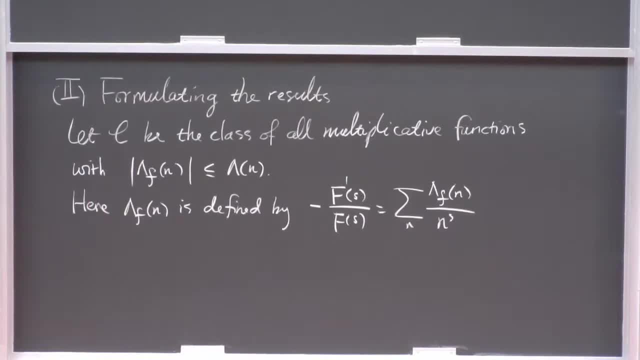 It also includes all one bounded completely multiplicative functions. OK, So before stating the result, I need a small definition. So we say that F satisfies the, A is equal voltage criterion. if this thing is true for all A cube co-prime. 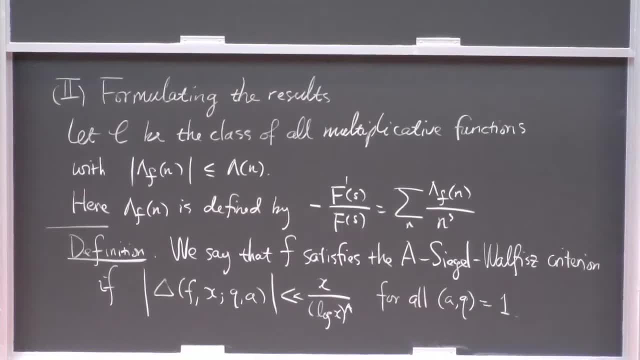 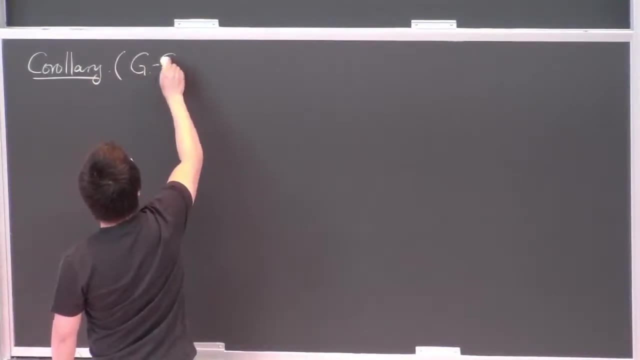 So, roughly speaking, the function is satisfy the A is equal voltage criterion if it's equity speeded modulo moduli up to log x to the A. So here is a corollary of our main theorem which is a bit easier to state. 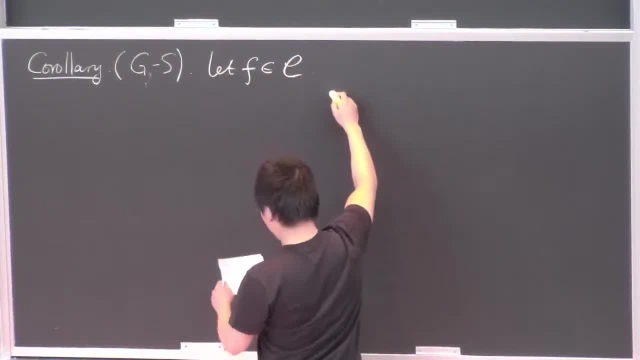 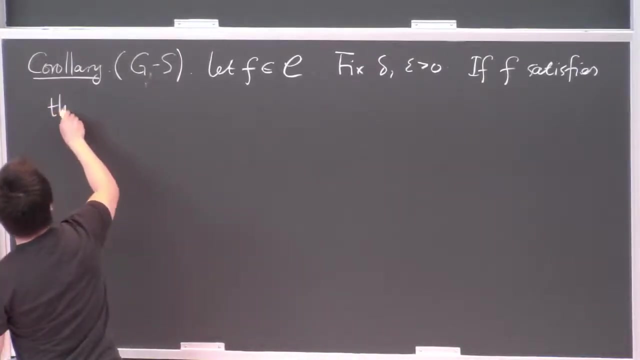 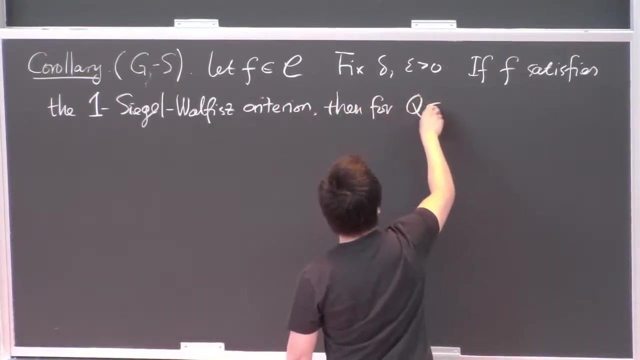 So let F be a multiplicative function, Fix two small constants, It's delta and epsilon. If F satisfies the one, the equal voltage criterion. then for Q up to x, to the one half minus delta, we have essentially the statement of the Bombier-Rivine grad of theorem for average. 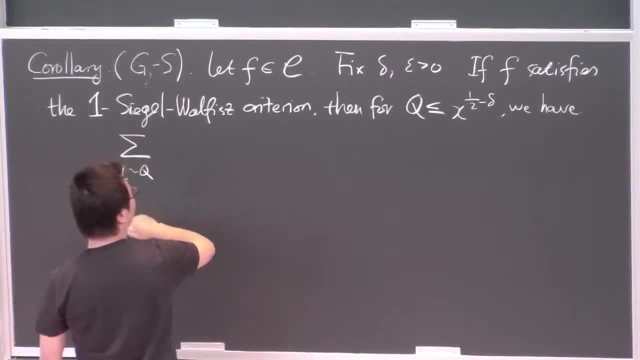 over moduli of size, capital Q. But now, instead of saving an arbitrary large power of x, arbitrary large power of log x, Okay, So we only save log x, Okay. So let me make two remarks, first about this assumption and then about this quantitative. 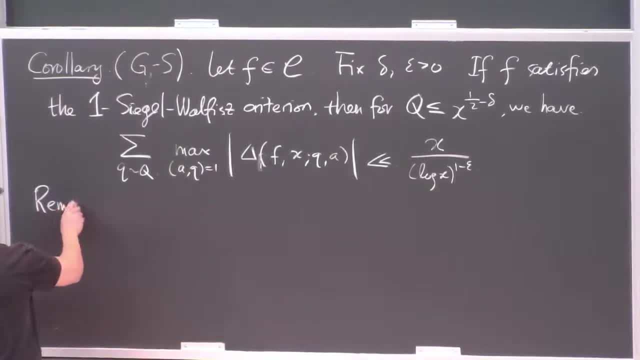 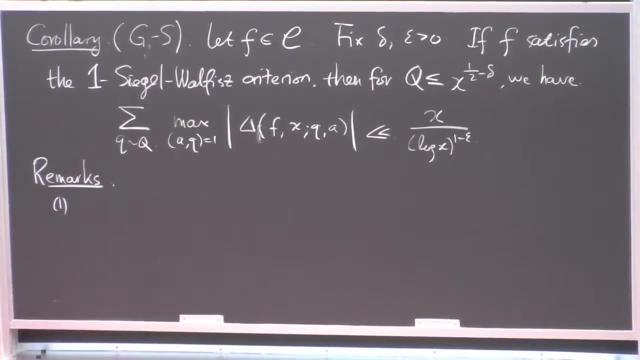 saving. So the first remark is trivial, That this criterion is necessary. So basically, if your F is a badly distributed modulo, a small moduli R, then for any Q that's a multiple of R this quantity will be large. So more precisely, if F is primitive character, chi mod R. 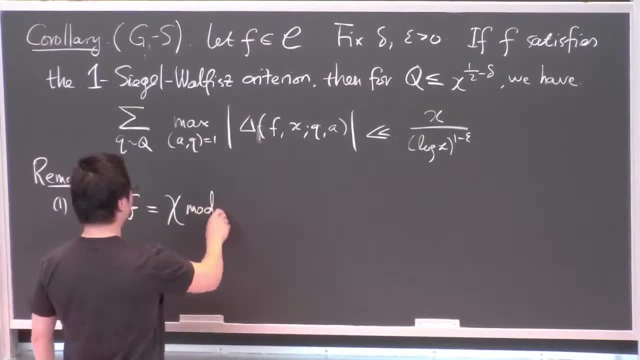 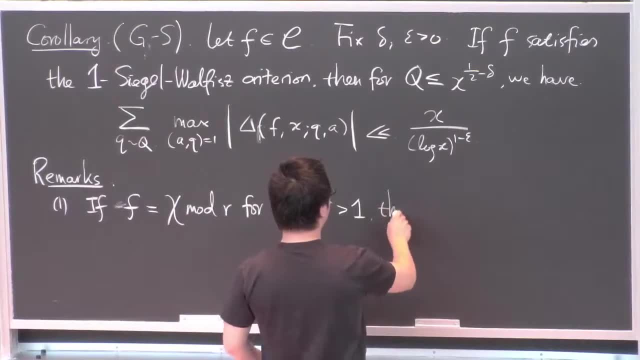 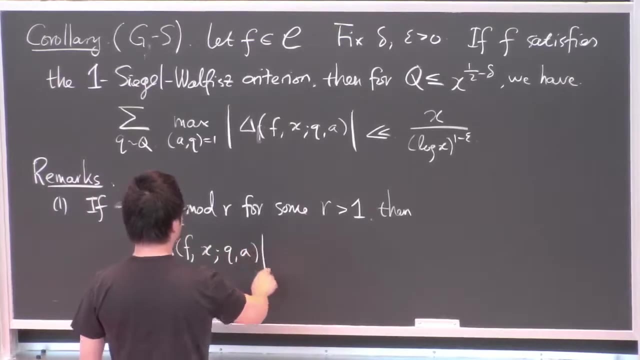 See Yeah, Chi mod R For some small R bigger than 1.. Then one can show that delta F x, Q, A is basically the same as the trivial bound x over phi of Q whenever R divides Q. Okay, Okay, Okay. 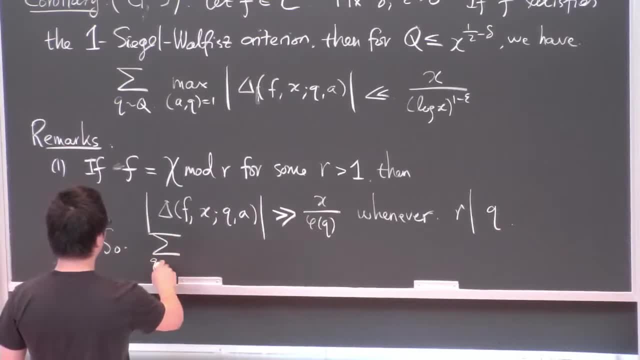 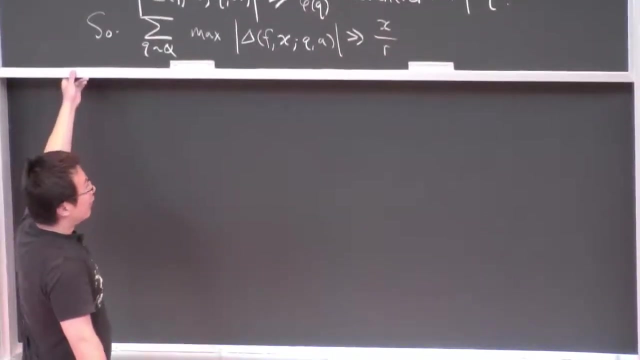 Okay, And this means that the sum will be bigger than x over R. So we have to rule out the case that the function is badly distributed, modulo, small moduli, And this is achieved by assuming the one Ziegler-Wolfish criterion. 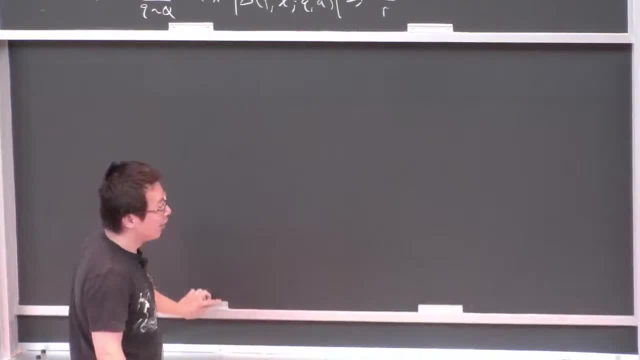 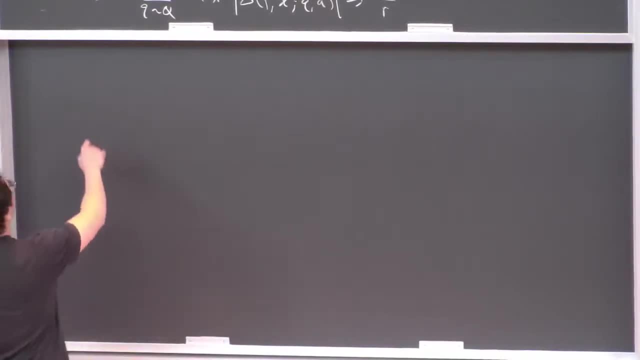 Okay, Okay, Okay, Okay, Okay, Okay. Let's we start with the one Ziegler-Wolfish criterion. The second remark is much more intricate- At least it was very surprising to us initially, which is that so you might think there are. 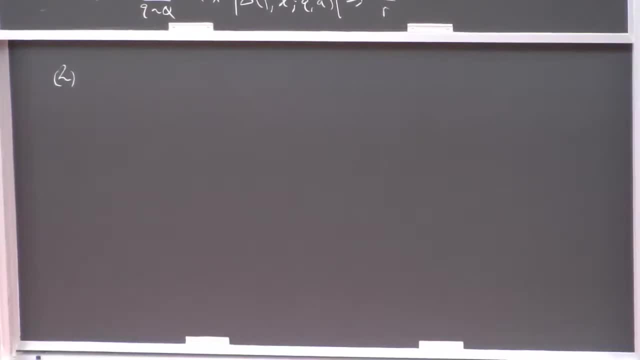 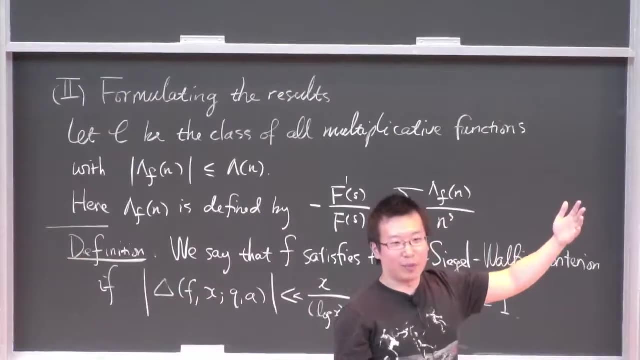 two- number one- appear twice in that statement: In the one Ziegler-Wolfish criterion and also in the one minus epsilon in the exponent. You might ask whether, if the first one is replaced by some larger A, whether one can replace the second one also by a. 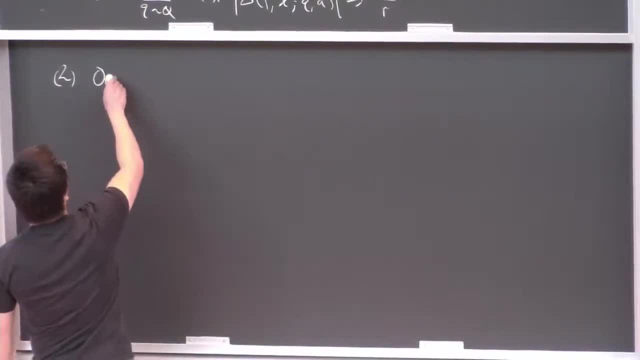 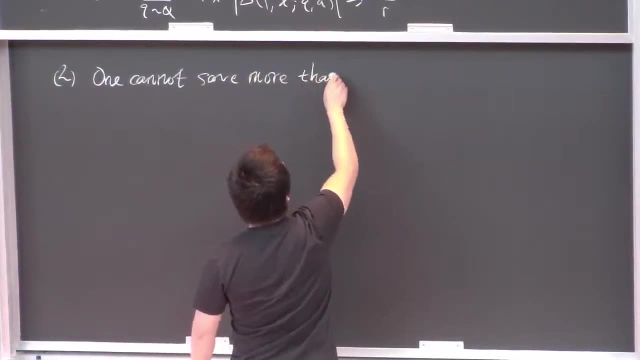 And the answer is no. One cannot save more than log x in general. So I'll give a concrete example here. but the basic reason is that when you study general multiplicative functions f, there are these primes that are between x over 2 and x, say. 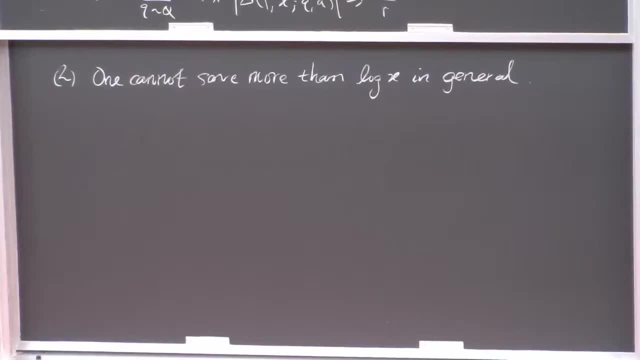 The values of f at these primes can more or less be independent and they can conspire in such a way that you don't have log x to the a equidistribution. So here is the example. Let p be the set of primes in a direct range, x over 2 to x. 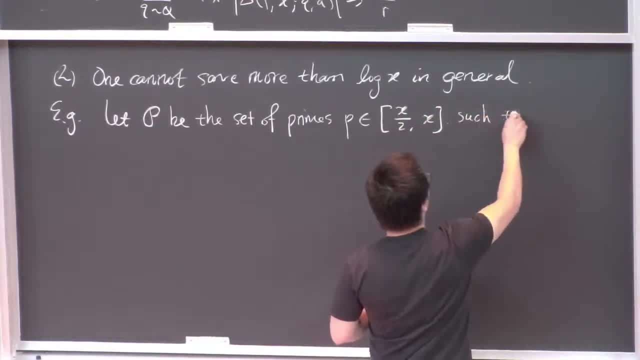 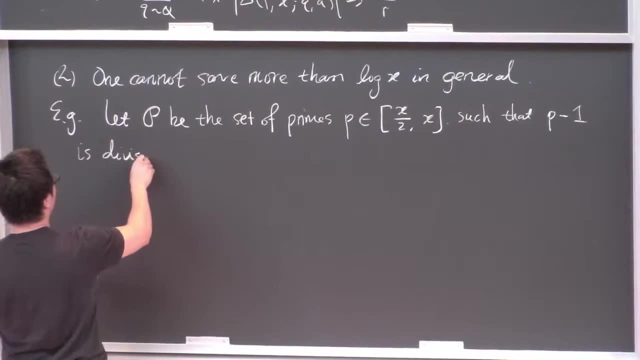 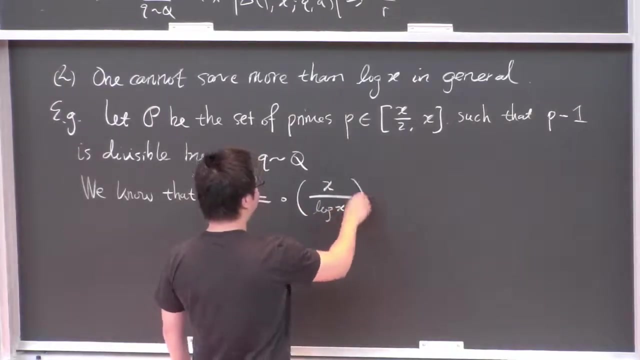 Okay, Such that p minus 1 is divisible by some q between capital Q and 2 capital Q. So we know that, and this is a deep result, The density of this set p is 0. So the size of p is little. o of x over log x. 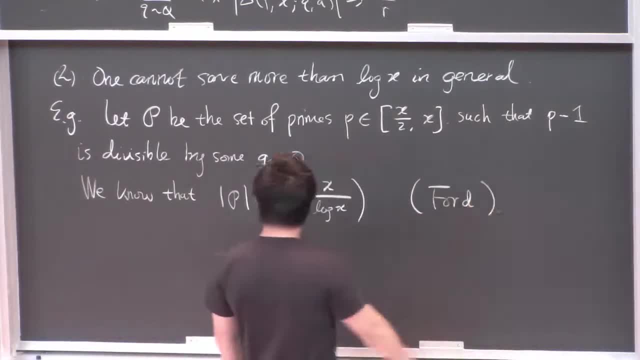 And this is a famous result of Ford. Now take my function to be the indicator function of this set of primes p. This is a multiplicative function because the values of f at these primes can be independent. Now if I look at delta, f, x, q and take a equals to 1.. 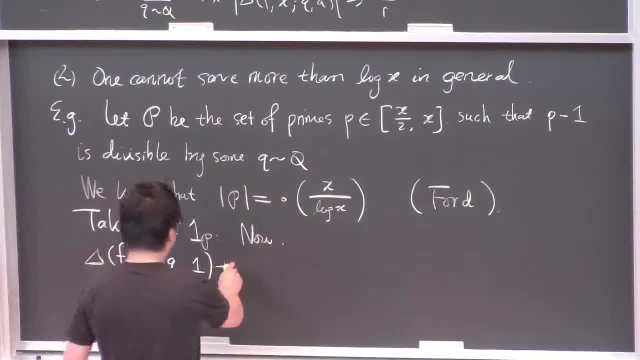 So look at 1 mod q. This, by definition, is the sum of the primes that are 1 mod q in p. So f of p here and f of p is just 1.. Okay, All right, Thank you Bye. The size of big Q. So the size of big Q can be anything that appears in the statement. 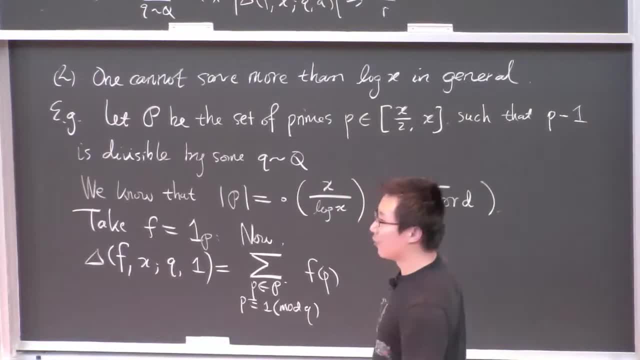 in the assumption of the corollary. So anything below X to 1 half minus delta will do For concreteness. you can take Q to be X to the 0.4, say So this is the right And subtract the expected main term. 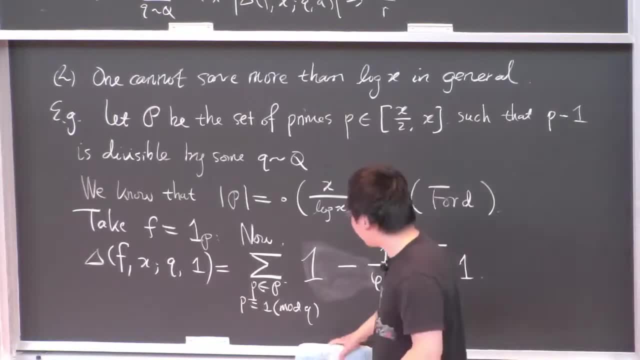 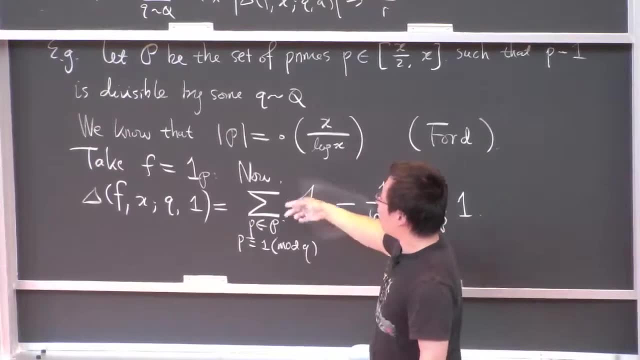 OK, so I'm going to do something bad in terms of board work. If you look at this first sum here, remember the definition of the set P. I can actually remove this criterion that P lies in the set script P, Because every other prime P satisfy the property. that P minus 1 does not have a divider Q. 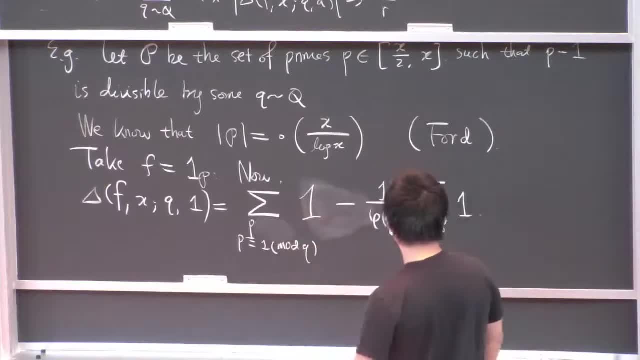 So they will not appear in the sum anyways, so I can just include it. And now, basically, the issue is that this is going to be much larger than that because of this estimate, And you can work it out to see that this is larger than the trivial bound. 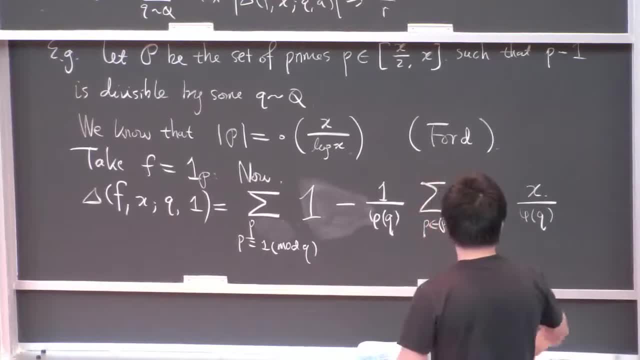 And so this is larger than X over log X times phi of Q, because this first term is about that size By the prime number theory in arithmetic progressions, assuming GRH. So OK, so this is not rigorous, but expect OK. 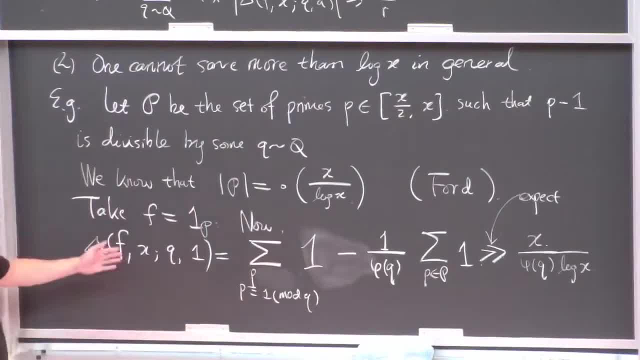 OK, OK, OK. So if you sum over all the Q, then you will see that the left-hand side of the statement of the theorem is at least X over log X. Any question about this statement and the remarks? OK, So now let me make a proper statement of a proper theorem. 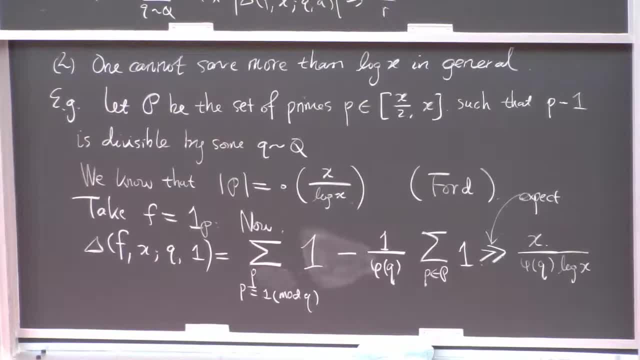 There seems to be some arbitrary assumptions in the statement of that corollary, in terms of assuming the 1-Zigal-Warfish criterion, for example, And that is basically because if you think about the definition of the quantity delta, F, X, Q, A- the expected main term may not be the correct expected main term for a general 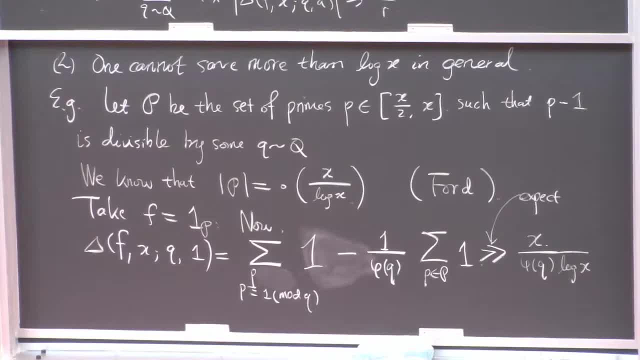 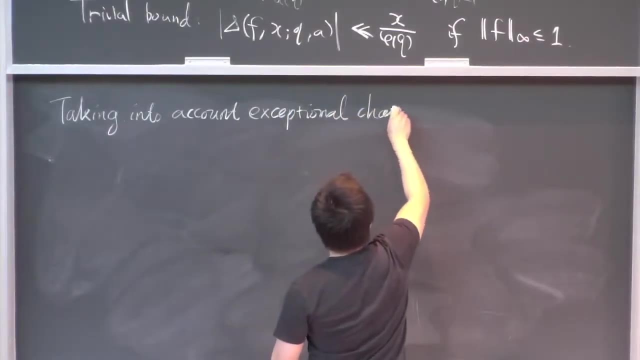 multiplicative function F. So to find the correct main term one needs to take into account exceptional characters. OK, OK, OK, OK, OK, OK. So if you think of, for example in the first remark over there, when F is chi mod R, you 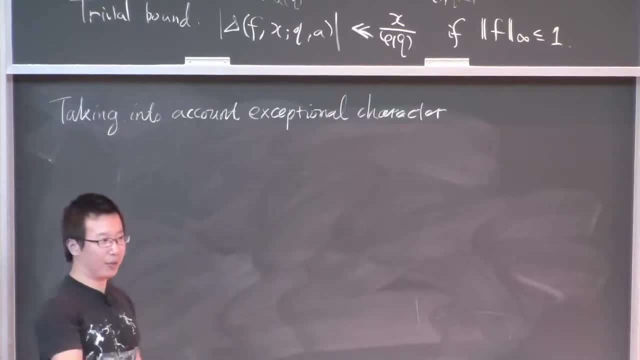 should think of the character chi be an exceptional character, Or similarly, when F is close to a character, then that is a bad character. We need to take that into account in defining our quantity. delta, F, X, Q, A, OK, OK, OK. 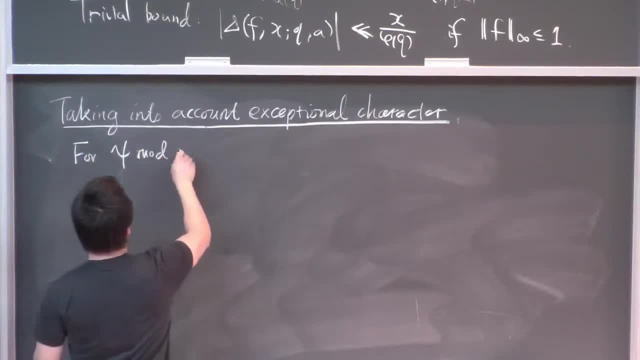 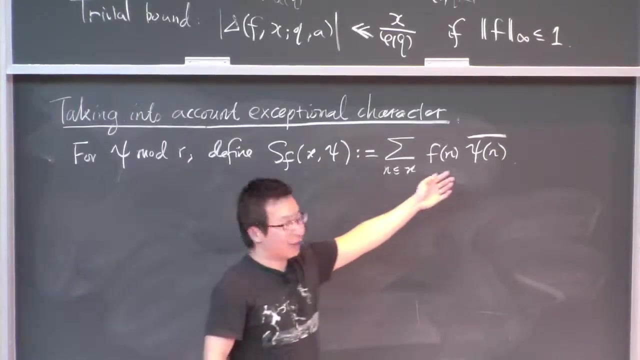 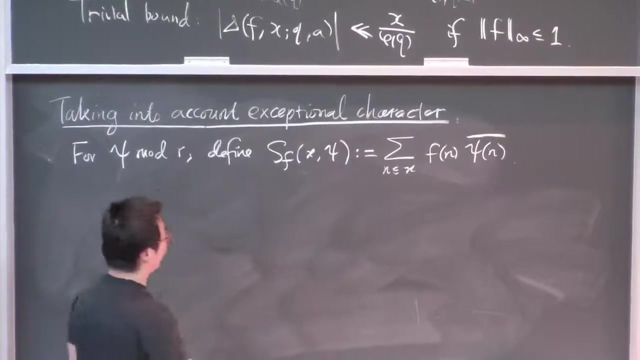 So for a primitive character of psi define the correlation of f with psi to be the sum of f, of n psi, of n bar, And so the exceptional characters will be those characters such that the sum is large. For technical reasons we don't quite look at this particular sum, but the following: 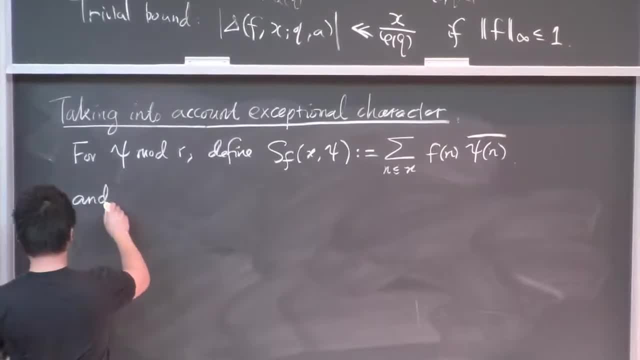 technical variance, But I won't say too much about it. So sigma, f, x, psi will be the similar thing, except that I allow this range to vary quite a bit. It's the supremum of capital, X, between x to the 1 half and x the usual sum up to capital. 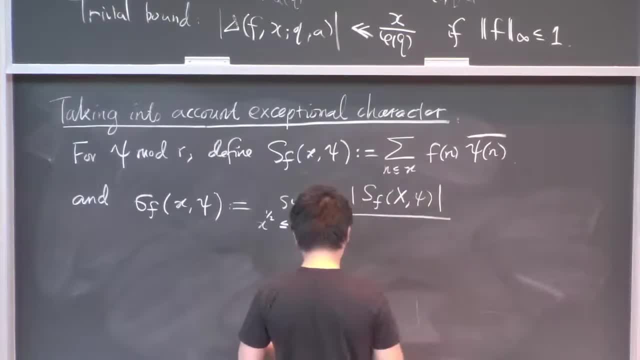 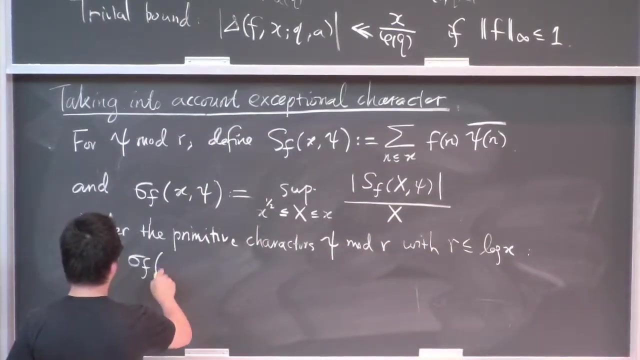 x. So it's scaled back correctly by capital X. Now I'm going to order the primitive characters: psi, mod r, with conductor r less than or equal to log x, according to the size of sigma f. So sigma f of x, psi 1, bigger or equal to sigma f, x of psi 2, and so on. 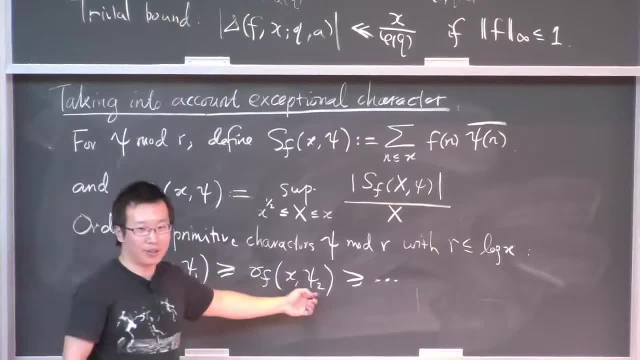 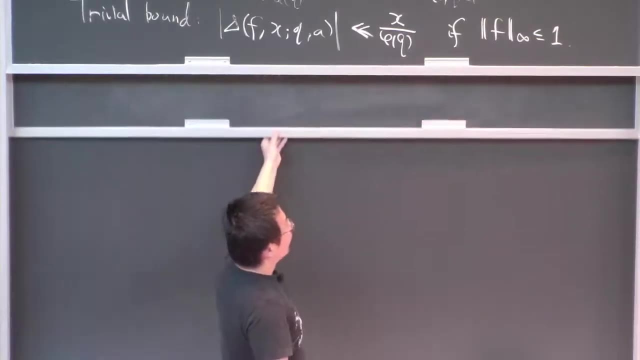 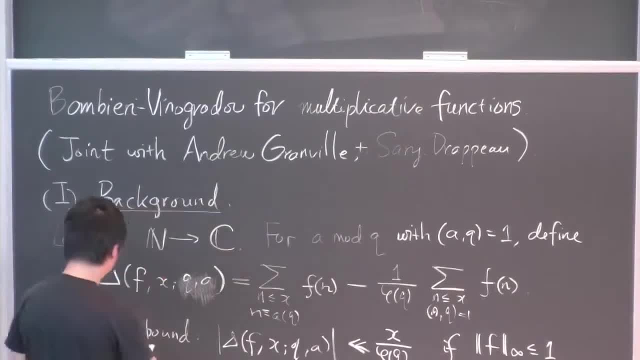 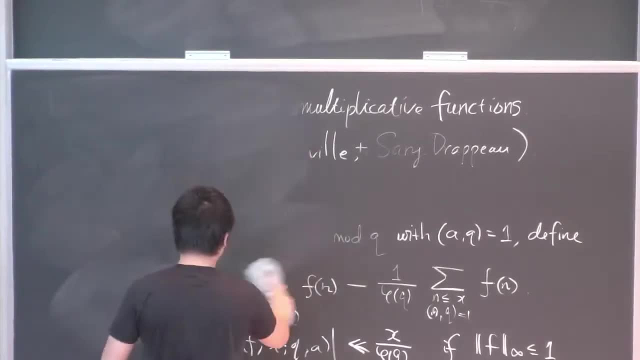 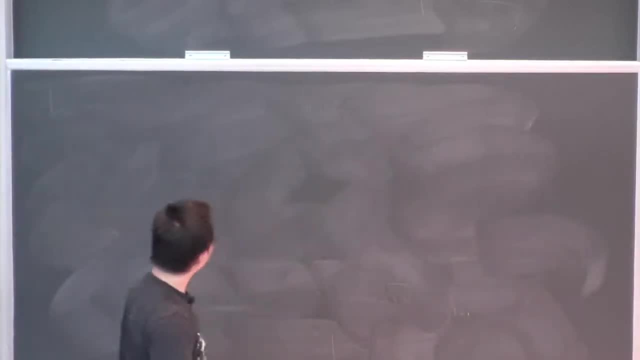 Yeah, Sorry, Sorry, We're assuming that the worst character is the trivial character. To see this, recall that the usual quantity delta f x, qA has the character sum expansion 1 over phi of q, sum over non-trivial characters, mod q and chi of A, Sf x, chi. 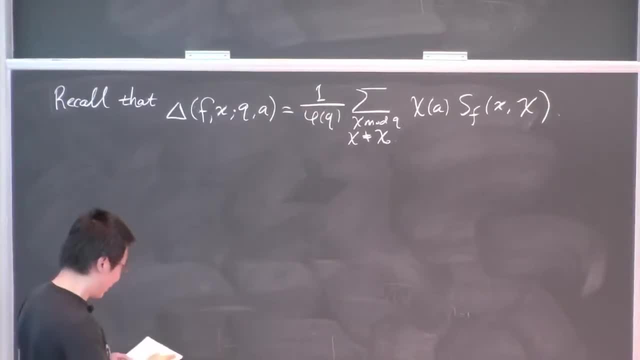 I hope my x and chi are different, but anyways, Now let's define for a positive integer k. Okay, So this is the quantity delta: k, f, x, qA. So this is going to be the measure of equidistribution. when you take out k, the k, worst guys, the. 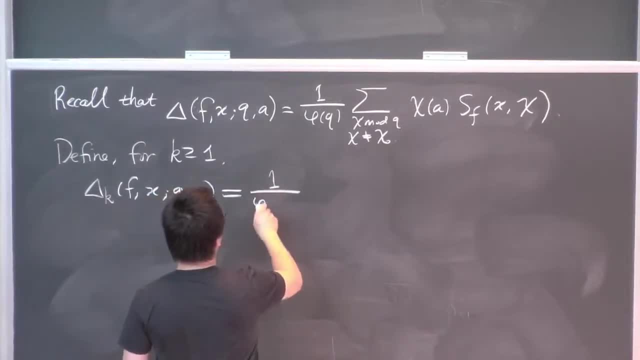 k worst characters. So this is the 1 over phi of q sum over chi mod q that are not induced by the first k guys up there. psi 1 up to psi k and the same sum and as above. So note that when psi 1 is the trivial character, if the trivial character is the worst guy. 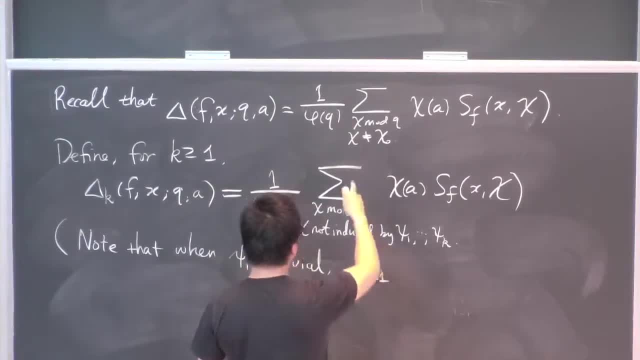 then delta 1.. Okay, So delta 1,, as defined on the second line here, is exactly the same as the usual delta. So the point of these two slides- sorry boards- are that we have the more precise capture of the main term so that we can expect this quantity, delta k, to be small without any further. 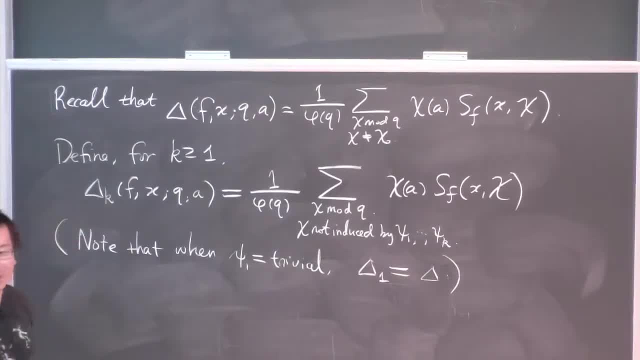 assumptions on the function f. Any question about this definition? So I haven't told any jokes yet, but some people are smiling, so I don't quite understand why. If there is anything wrong, please let me know. Sorry, Who is that? 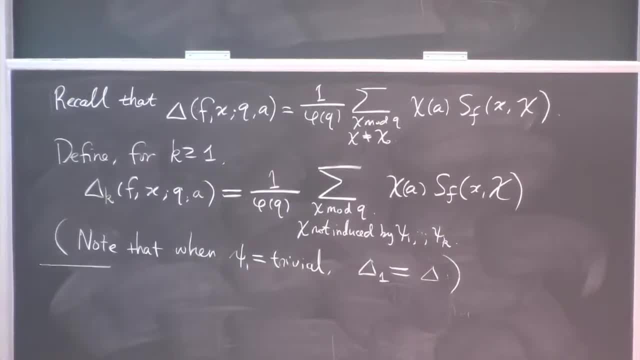 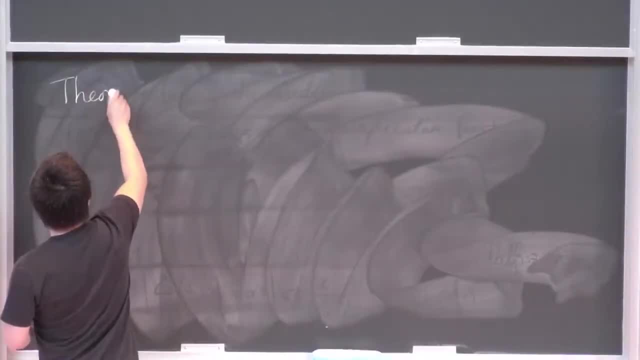 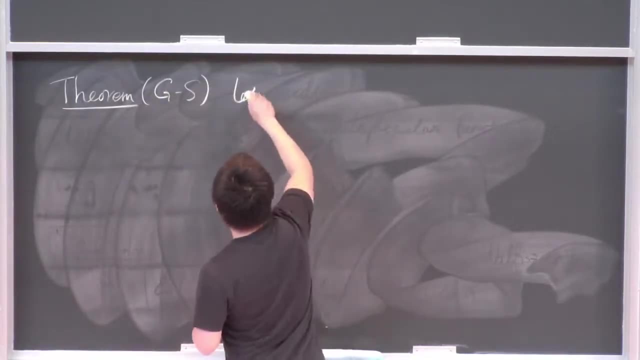 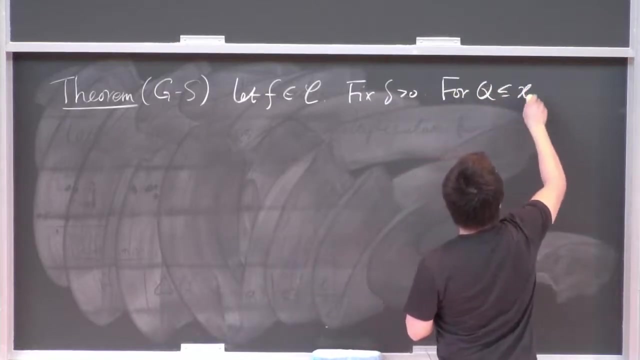 That will have that corollary as a corollary. So again, let f be our multiplicative function. Okay, function and fix on delta For Q, for capital Q up to X1, half minus delta, we have the following bound: 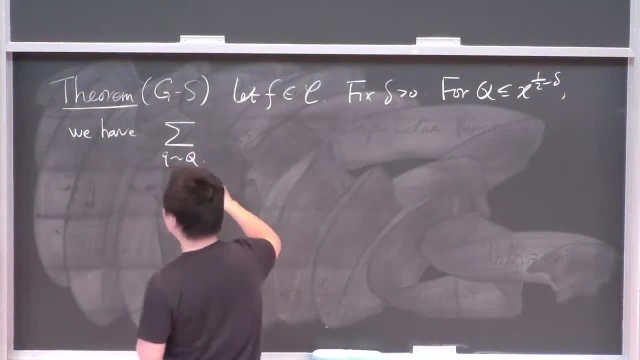 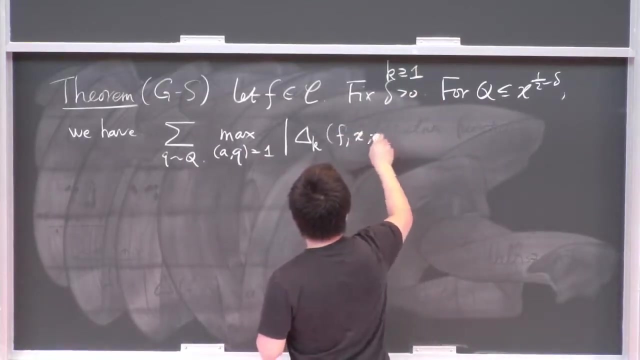 If I sum over moduli Q of size, capital Q. OK, so I also fix positive integer K here along with delta. So if I look at delta K, then this is small on average. More precisely, you save log X to the power of 1 minus 1 over square root of K plus 1. 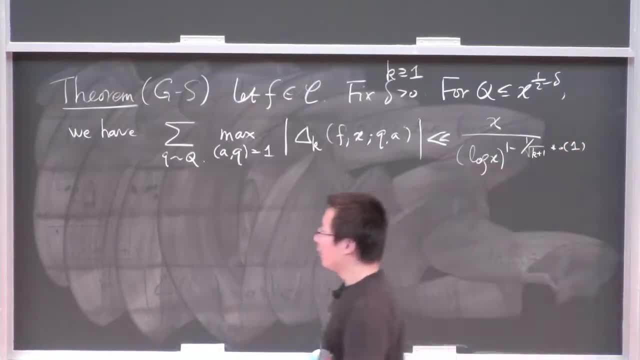 plus little over 1.. So, roughly speaking, the corollary follows from this theorem by taking K to be arbitrarily large. So I won't talk too much about this exponent, but let me just say that. So there is work of Grandview, Harper and Sound. 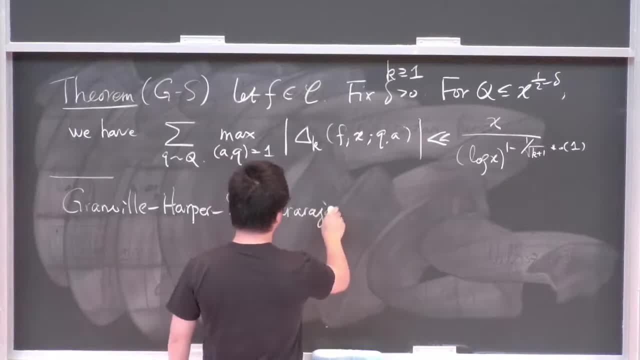 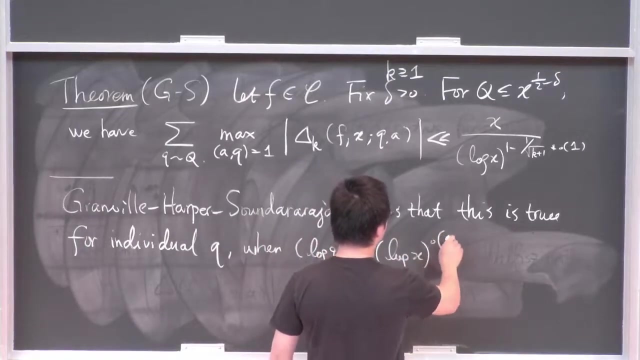 They showed that this is true for individual values of Q, when Q is small, for individual Q, when log Q is log X to a small power. OK, So there is a small power And this theorem will get the same type of saving on average over Q and over a much wider 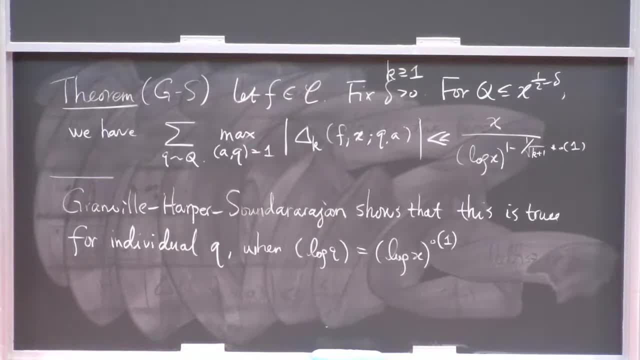 range of Q. Yeah, So is that little Q? between big Q and 2 big Q? Yes, OK, Can you get between 1 and 2 big Q, or do you need to restrict it like that? No, no, no. 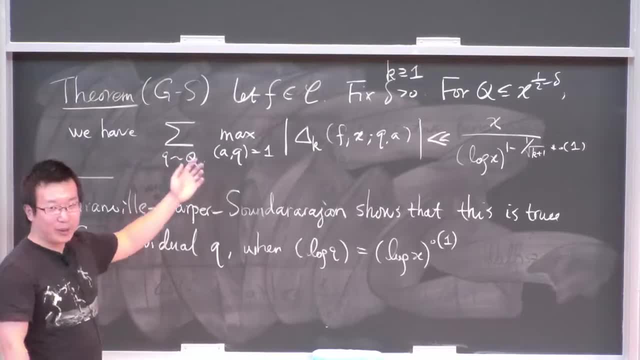 OK, Yeah, So that's a good question. So I kind of avoided this delicate issue you just mentioned. So this is certainly the result, And if you can get the average over all moduli between 1 and capital Q by just summing over, 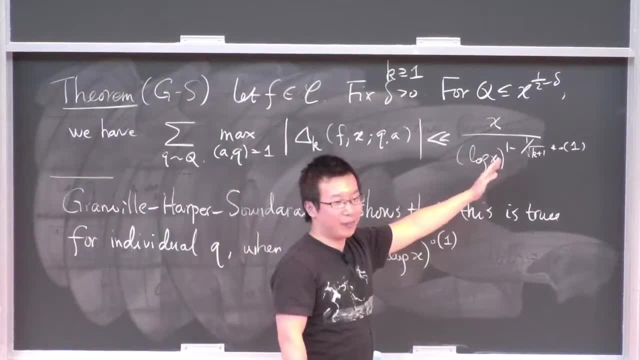 this diadically, But the thing is that you will lose. the trivial bound is no longer X anymore. The trivial bound becomes X, log X. So it looks less nice. That's why I wrote it this way In the usual. it doesn't matter, because you save an arbitrary power of log X anyways. 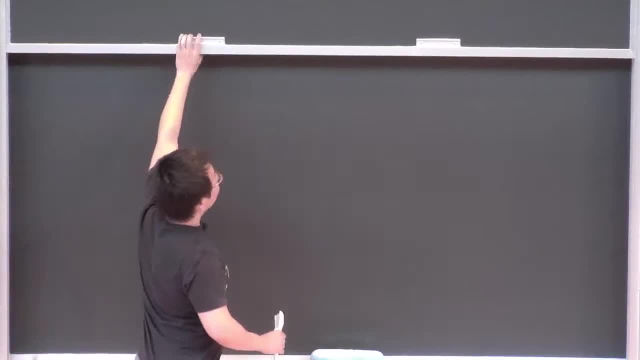 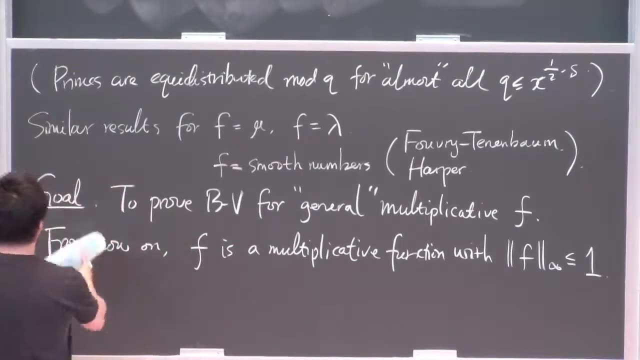 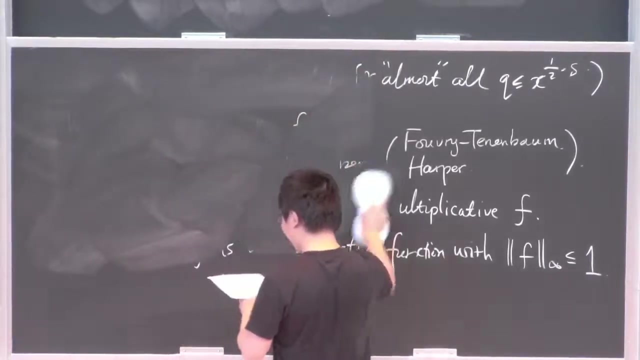 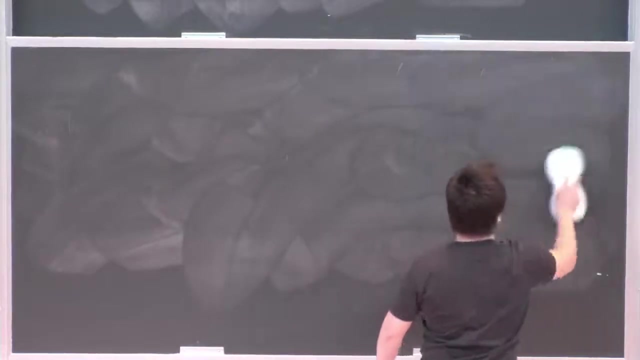 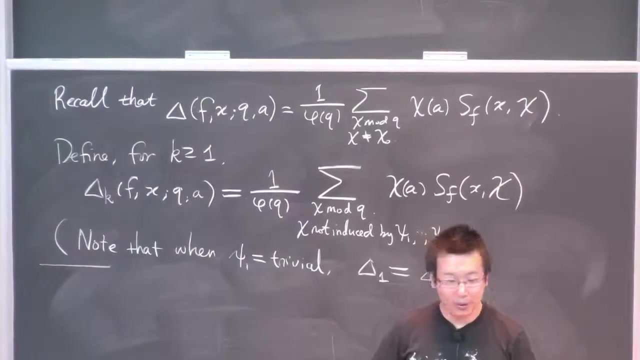 Yeah, thanks, Yeah, Thanks, Bye. Okay, so in the next, in the last, however many minutes of my talk, I would like to first of all just give you some idea into the proof of this theorem, and then I will talk about. 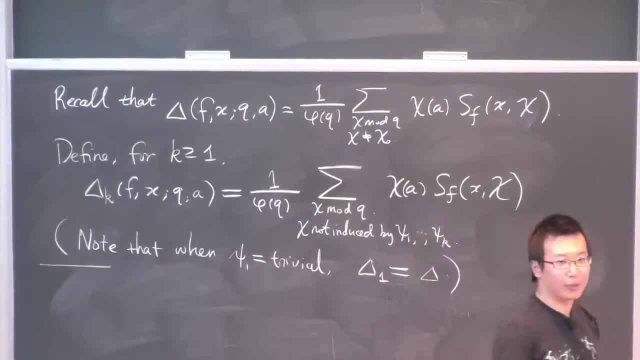 some similar results that trying to understand these issues better. So before I start I should just say that for the classical Born-Beer-Rivenogradov theorem we now know many proofs of it. Perhaps the most modern proof is to use Volant's identity to arrange things into a bilinear. 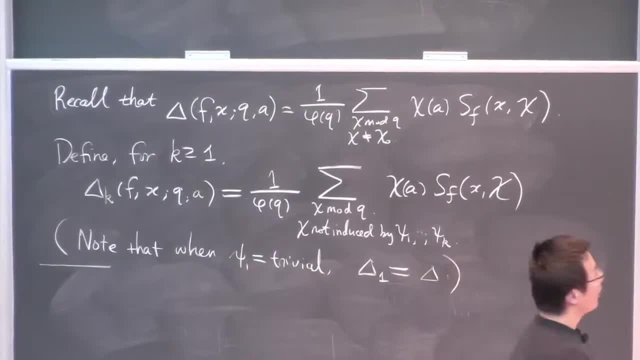 sum and then use the large sieve. Now it doesn't. we don't know how to adapt any of these existing proofs of the Born-Beer-Rivenogradov theorem in this setting, because, for example, for a general multiplicative function f, we 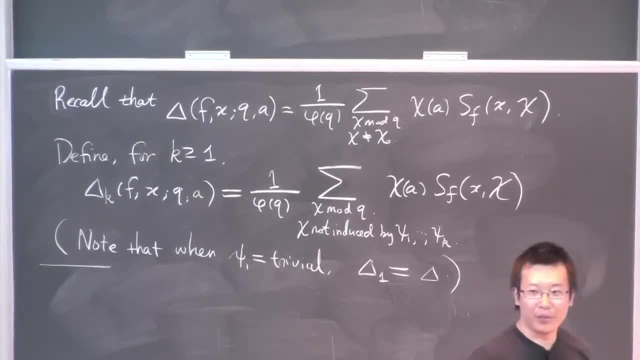 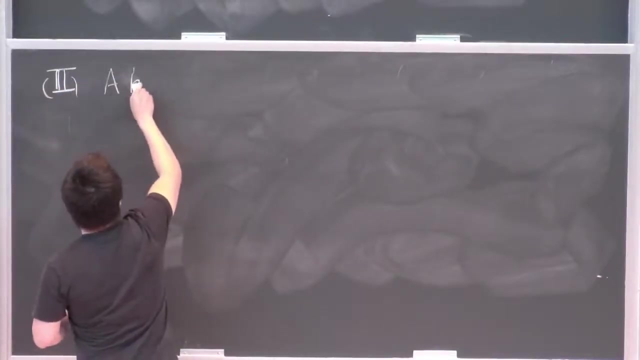 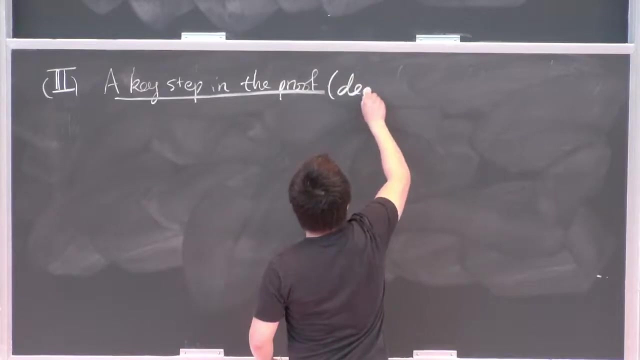 don't know how to arrange things into a bilinear sum, So we achieve that part of the argument in a slightly different way, and this is what I'm going to talk about. So this is the key step in the proof, And this step allows us to deal with a large module, a. 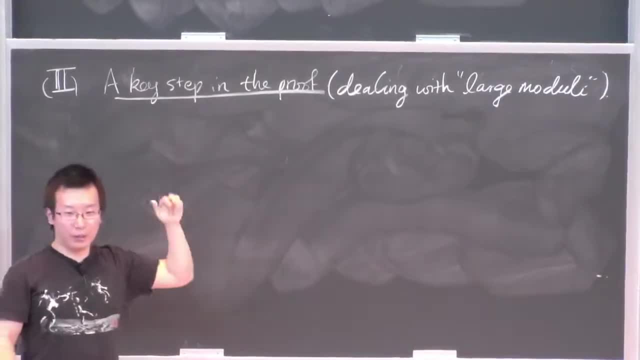 So the rough strategy is that the theorem of Granville's, Harpo and Sound deal with small module a, and the step I'm going to talk about is going to deal with large module a on average. So just one piece of notation for this problem. 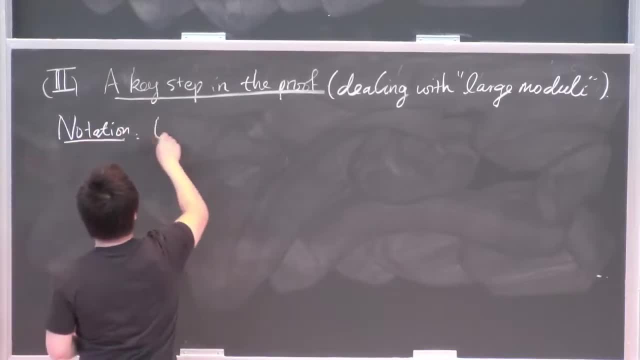 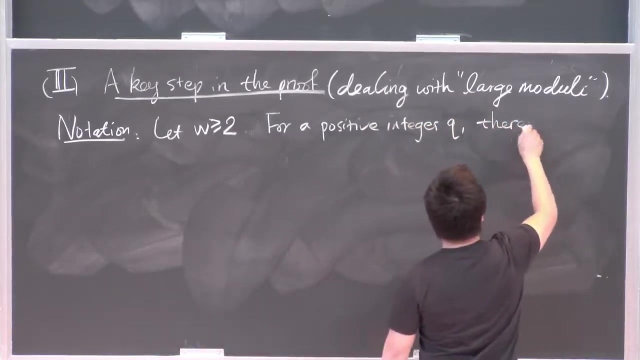 I'm not going to get into it too much because I'm still just using support over and over it section. Let w be a parameter, at least two, For a positive integer q there is a unique decomposition. q equals to qr times qs. R stands for rough, S stands for smooth, So 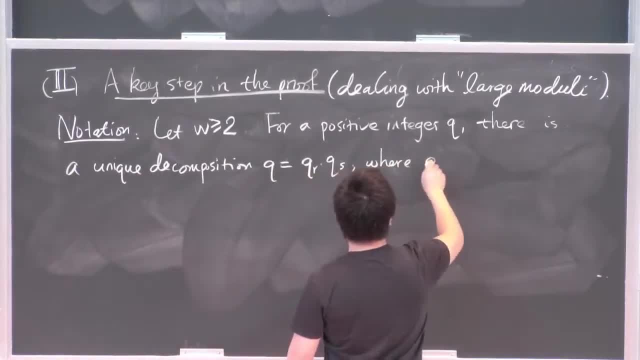 qs is the smooth part of q, So qs is the yeah. So you factor out all the prime factors of q, Everything that's at most w put it to qs, Everything else, put it to qr. I hope that's clear. And here is the proposition. 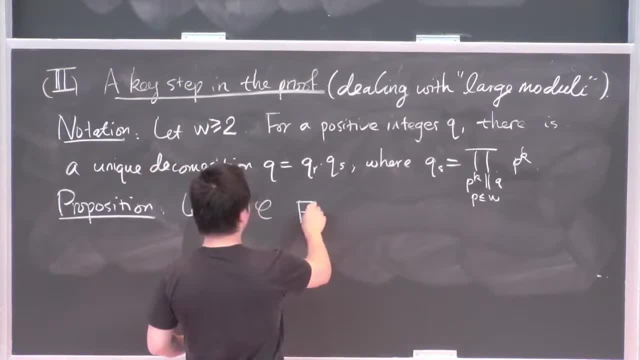 Let f be my multiplicative function And fix delta For q, for capital, Q up to x to 1 half minus delta we have. So the statement is going to be similar as before, except that, except it's different, Different in the sense that 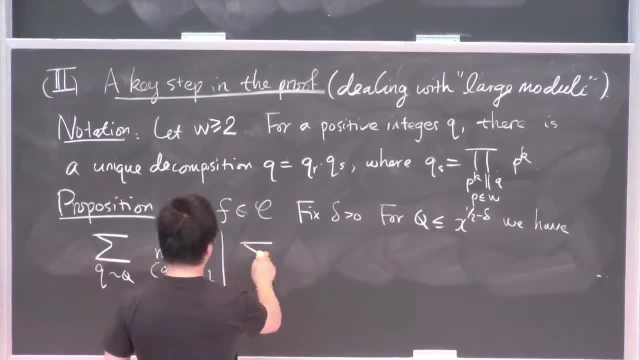 it's easier because there would be a more complicated main term. So, as before, I'm looking at sum of f of n over a mod q, But now I'm looking at the main term that basically takes out the rough part of q, So 1 over qr, sum of n up to x and congruent to a mod qs f of n. 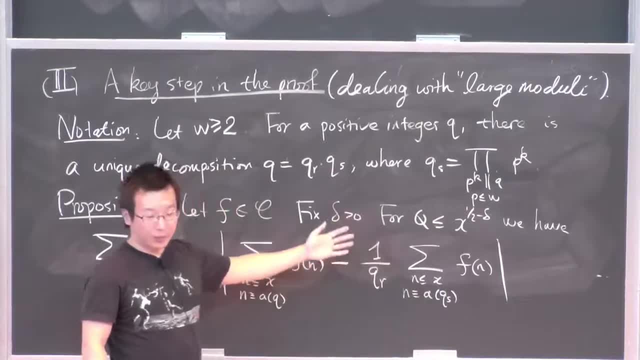 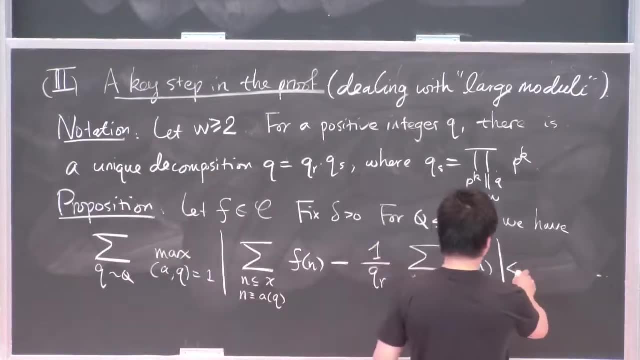 So if you think of this as an adjusted main term that deals with the rough part of q but not the smooth part of q, And this we can bound Bounded by x over w, to the 1 half plus log log x over log x. 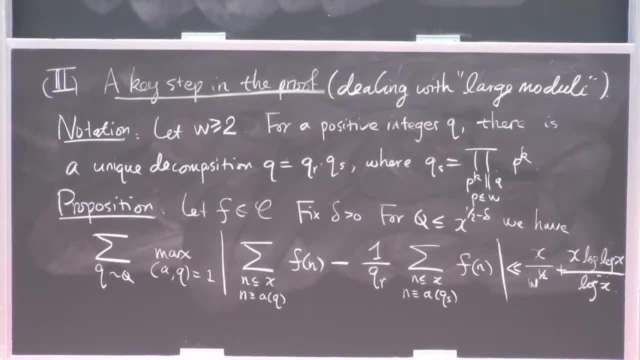 Ultimately, the May theorem is going to be deduced from this proposition. I'm not going to go through that, But in a very, very rough sense, what's happening is that this proposition allows you to look at just these things, things that have smooth moduli. 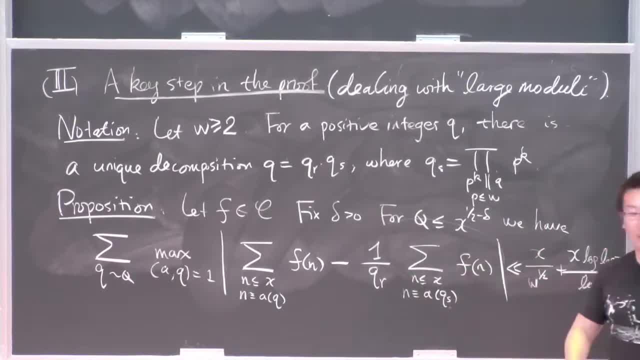 And most of the smooth numbers will be small. So you will be looking at mostly small moduli And that reduced to the case of Granville-Harpoon sound result. Yes, Is there a range on w? Yeah, w can be anything in this statement. 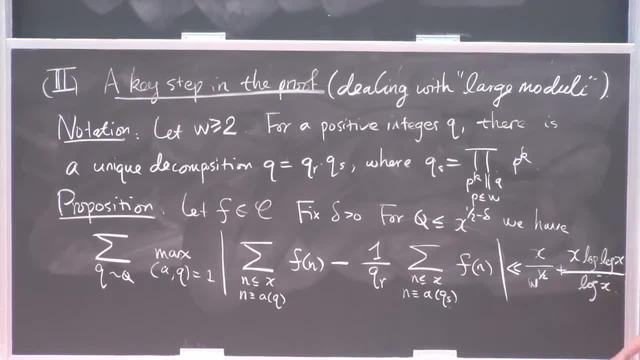 So, of course, the most logical choice of w would be something like log x squared, Because if you choose w to be larger, you won't get any better bound because of this term, And if you choose w to be too small, this bound will not be good enough. 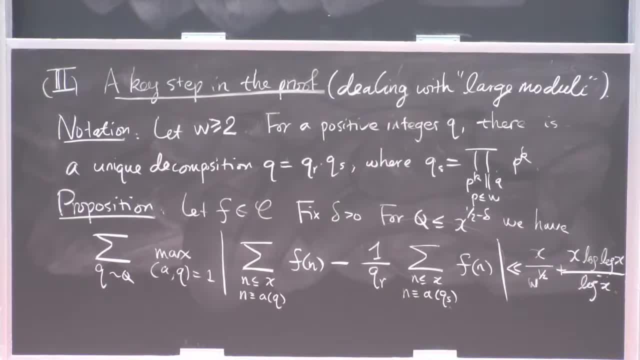 But the proposition as stated works for any w at least too OK. so I'll spend 10 minutes to give you an idea of what the idea in the proof of this proposition is. But let me just mention that, for example, for if I'm only interested in the average, 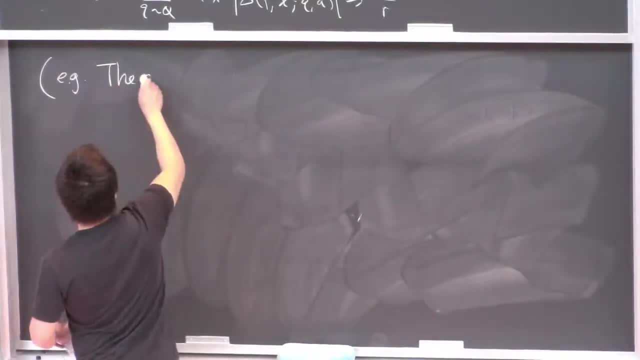 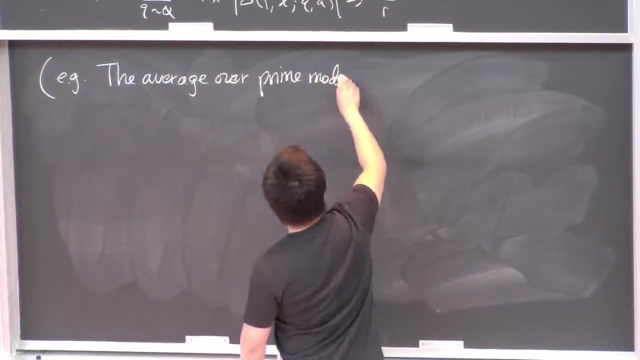 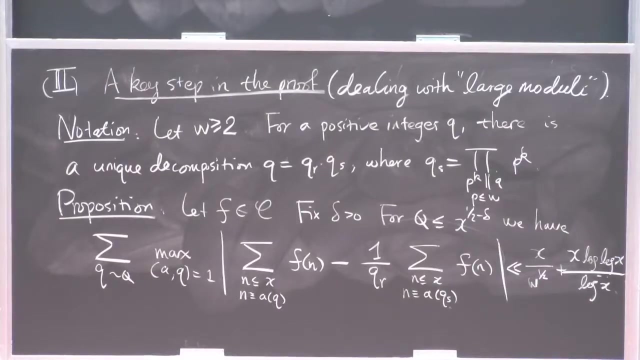 of a prime moduli. So if q is prime, then the qs is just 1, which means that this quantity is precisely delta fxqa, And let's just go back to our familiar quantity. So in this case, the average of a prime moduli, q, for this type of proposition was worked. 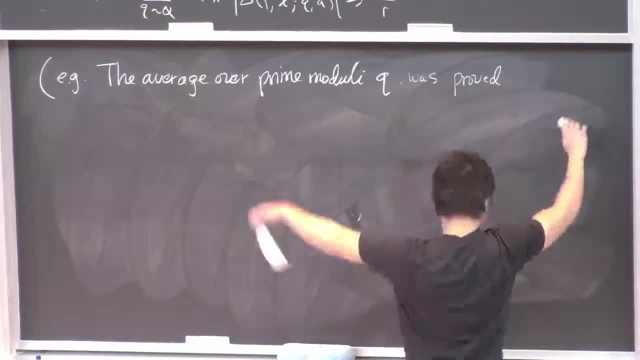 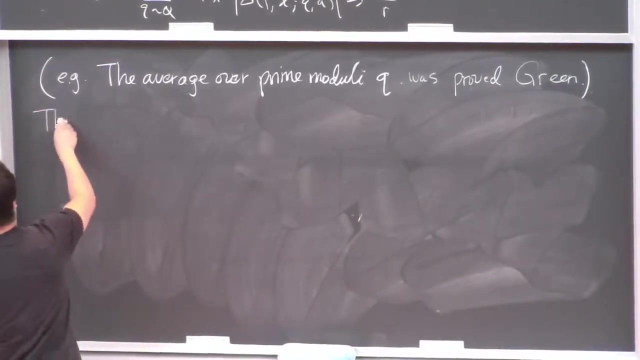 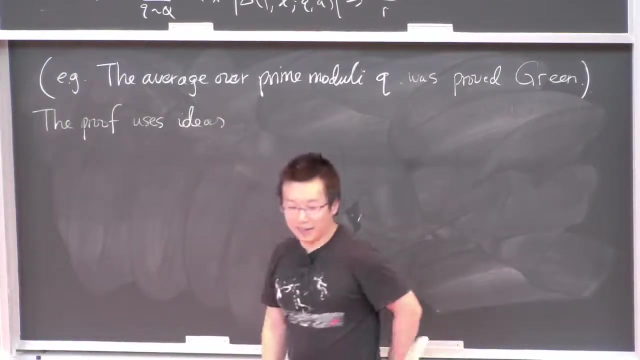 out by was proved by Van Green in a recent work. That was not a joke, OK, and so I also know that this is recorded. so I need to mention a lot of names. So the proof uses ideas that go back to a lot of people. 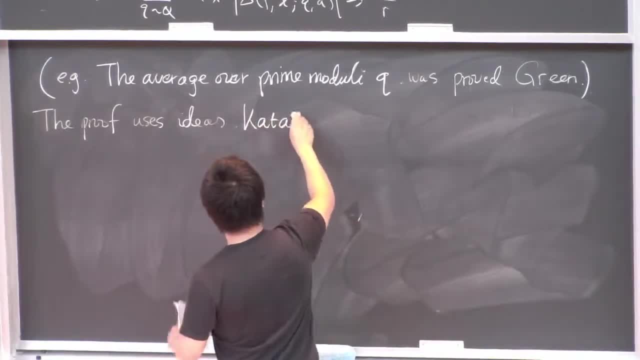 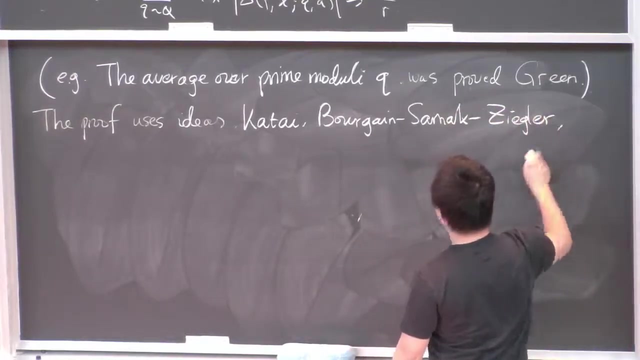 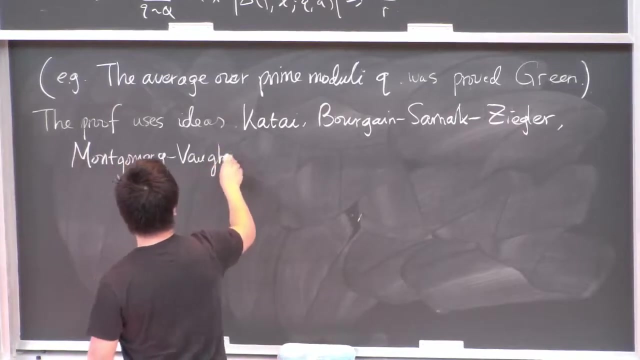 So sometimes this is referred to as the Katai And in the more classical analytic number theory literature methods of this type also goes back to a work of Montgomery and Volan on exponential sums with multiplicative functions. OK, Thank you, Thank you. 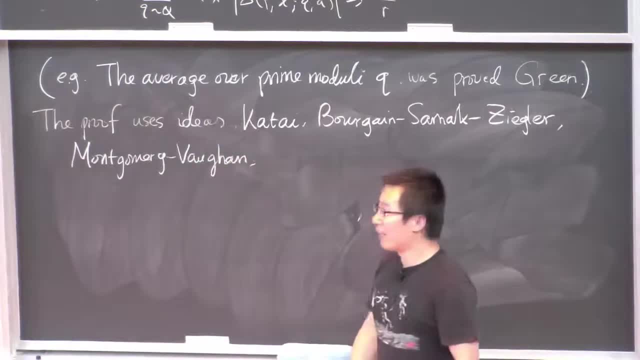 And then the last few years. we now know that to get these kinds of more quantitatively superior bounds, we use a trick or identity of Hamahi, And this also appeared in the recent work of Matamagiride, Ziwei and Tao about multiplicative. 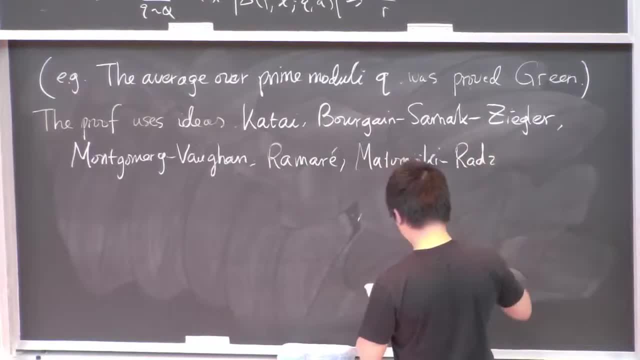 functions in short intervals. Last but not least, there is this work of Van Green that applies this method in contact very similar to ours. Having got these out of the way, I can tell you what the idea is. To start with, let's choose. 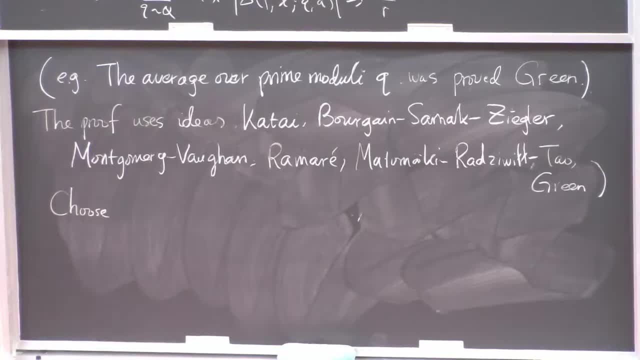 I want to get rid of this maximum thing and the absolute value thing. So choose xi, q and aq mod q, such that that maximum thing and the absolute value thing is achieved When I, The residual class is aq, with the phase xi q. 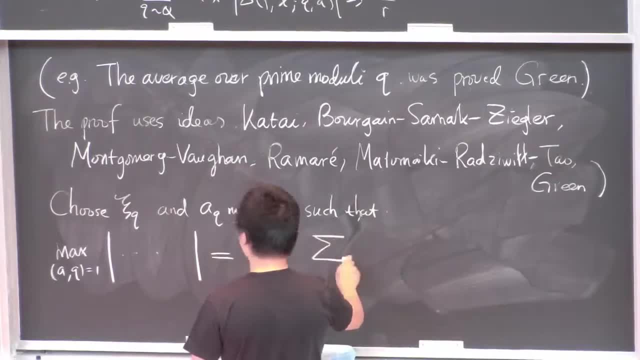 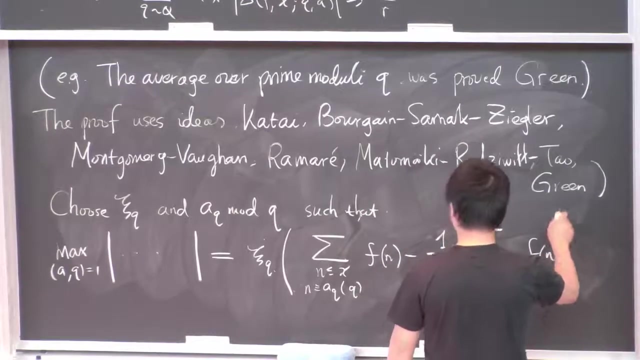 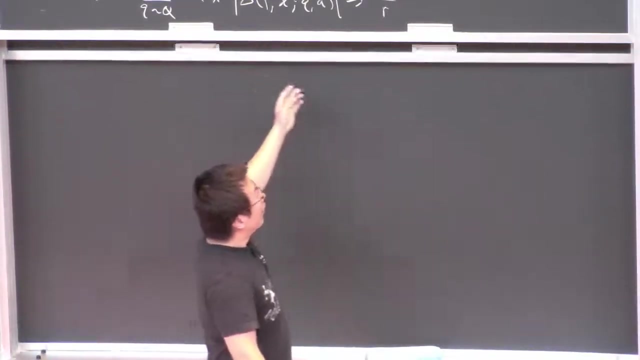 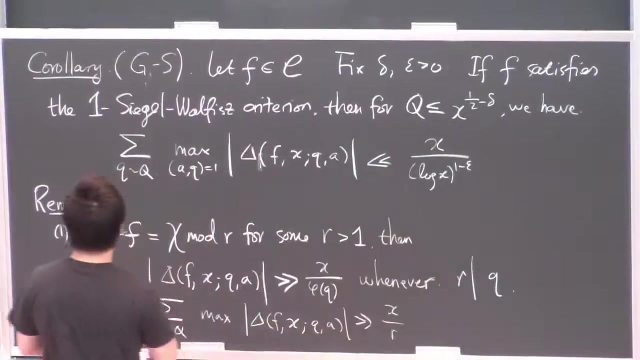 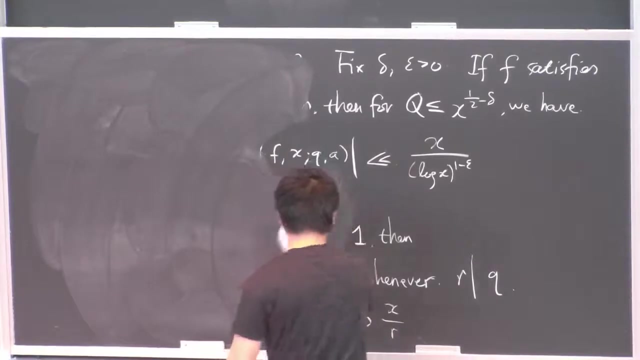 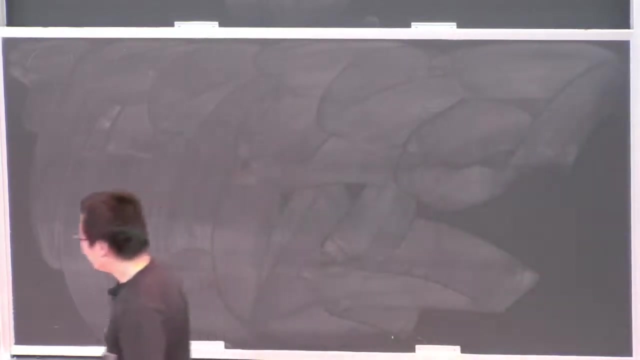 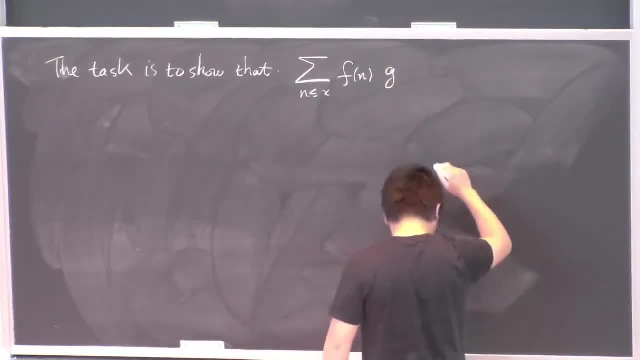 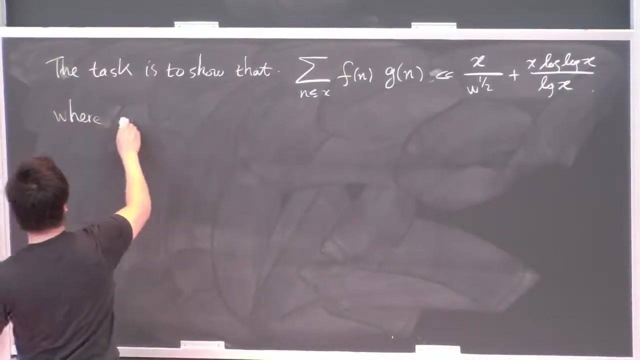 f is orthogonal to the function g that I'll define in a moment. So the function g is precisely what you will get if you unravel what you want to prove. So g is the sum over moduli q, xiq, the indicator function of n congruent to aq mod q. 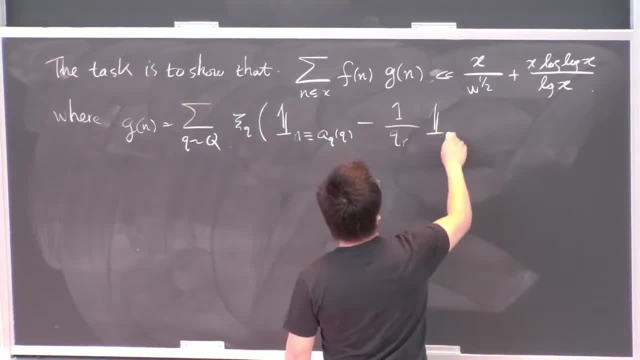 minus 1 over qr, the indicator function of n congruent to aq mod qs. So the point is that f is this mysterious multiplicative function that we want to understand, but we only want to understand that it's orthogonal to this, more concrete and combinatorial in nature. 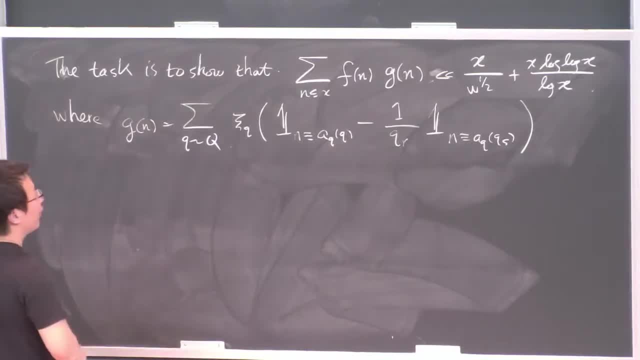 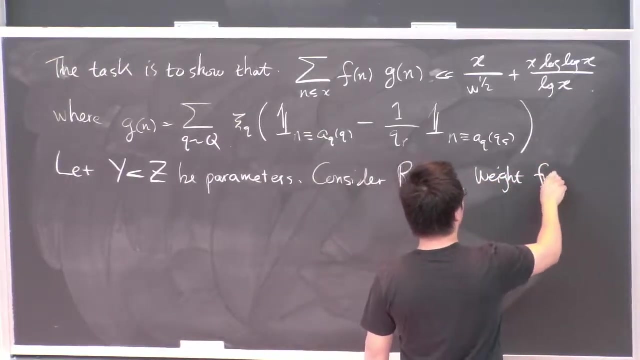 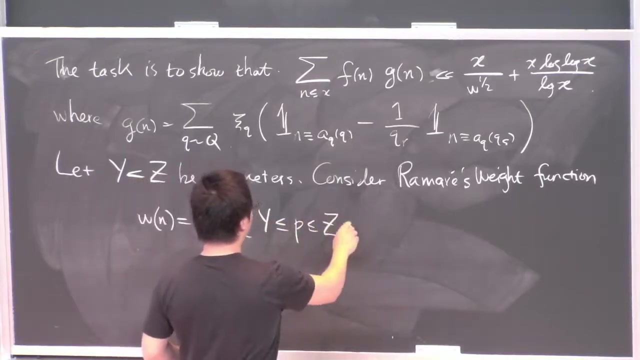 the function g. Basically, you want to get rid of f and we want to just study g, So let y and z be parameters. Consider the weight function introduced by Hamahi. So y and z, which is the number of prime devices in the range between y and z of n. 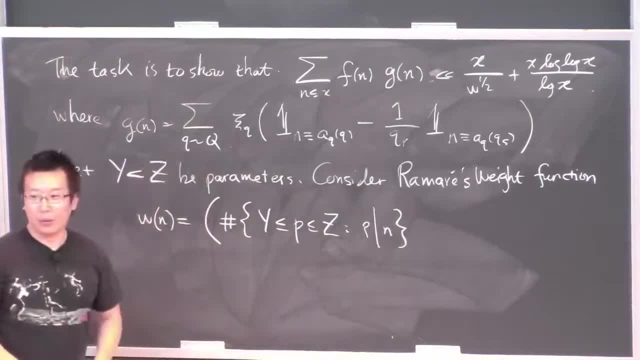 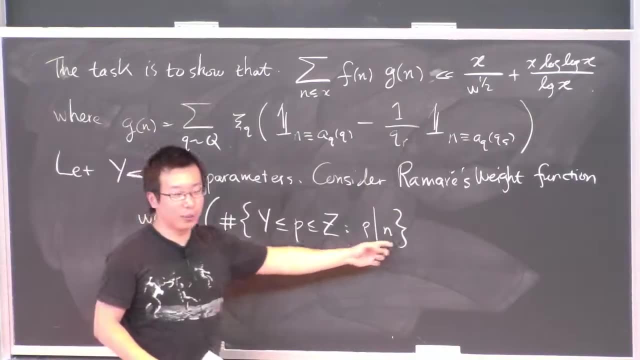 So that's the number. So you should think of y to be some power of log x and z to be a small power of x, something like that, so that you expect this quantity to be something that goes to infinite Plus 1.. 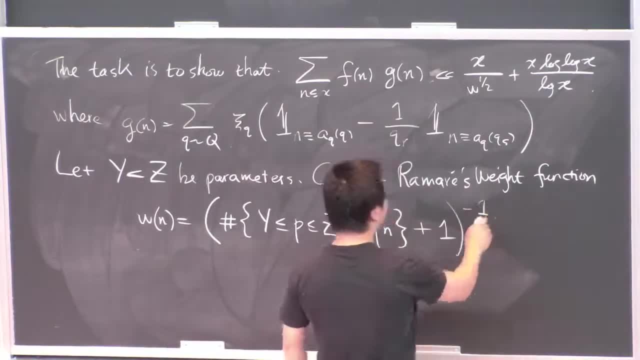 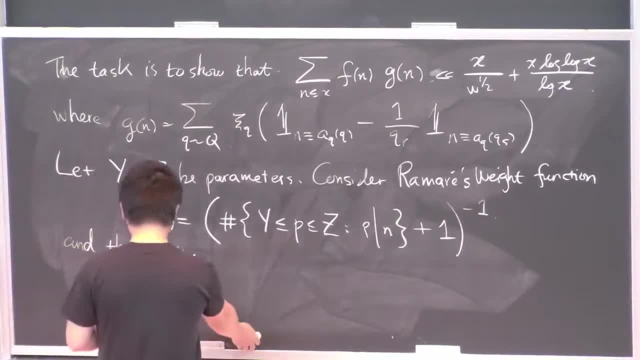 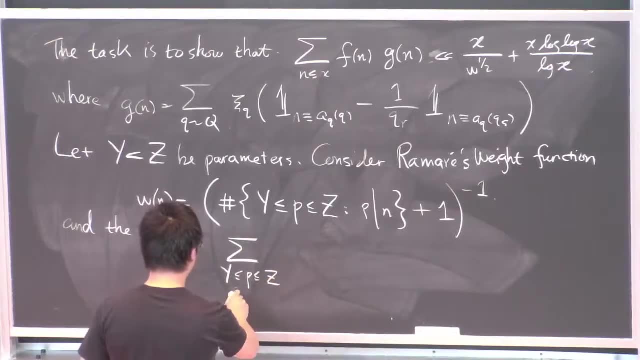 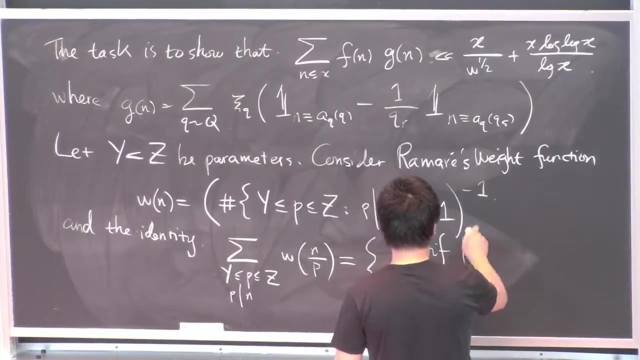 Question: Question. So the following identity I sum over primes between y and z that are a prime factor of n, of w, of n over p. This is either 1 or 0.. It's 1 if n has a prime factor. 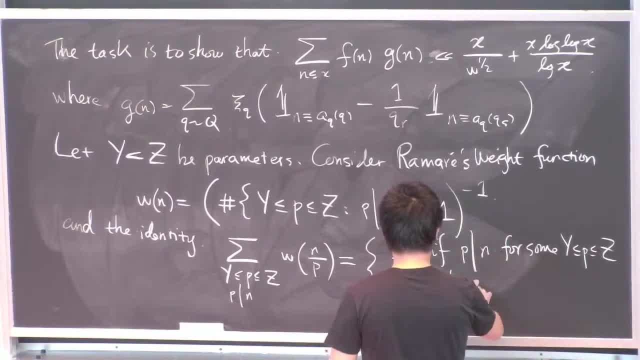 And 0, otherwise Otherwise Also. the other way about this is also 1.. 1 means that the prime factor is less than or equal to 1. if n has a prime factor of n over p, that's the first one. 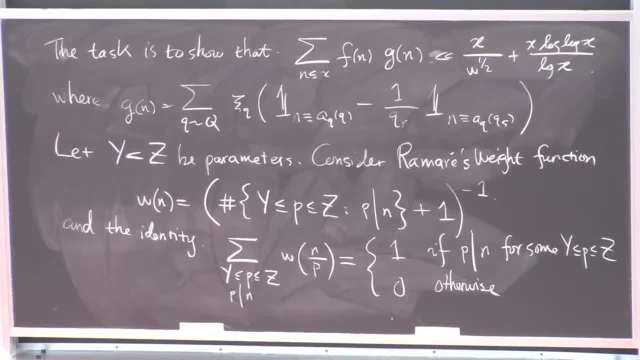 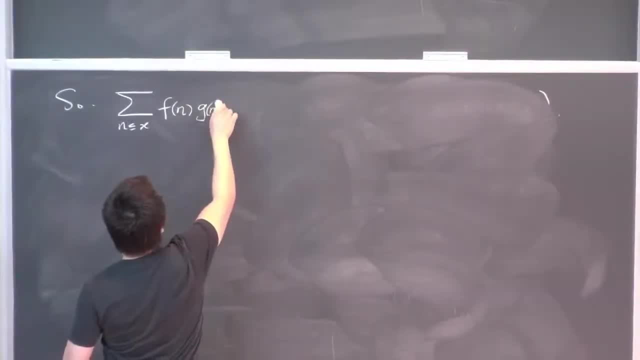 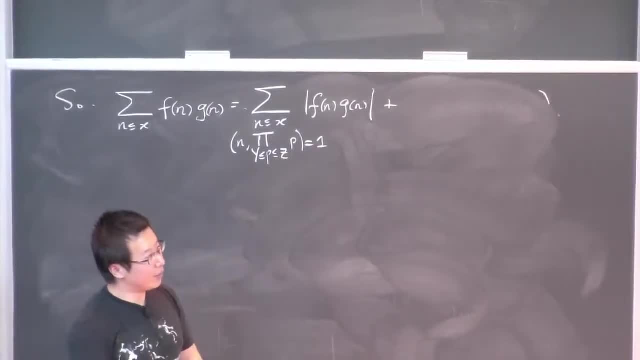 the case when my n has a prime factor in the correct range, I use the identity. OK, So the first term can be bounded just trivially by x times. OK, So the first term can be bounded just trivially by x times using a simple upper bound CIF And this gives you the log log x over log x bound in. 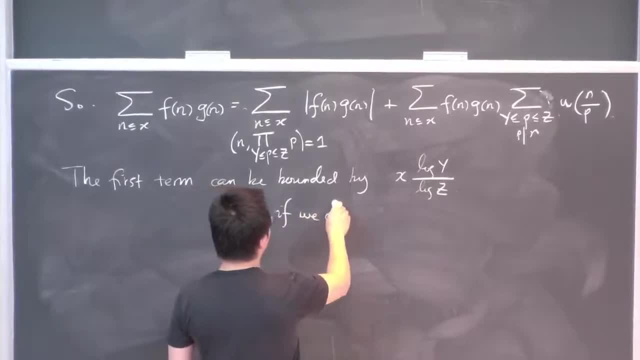 the proposition if we choose y to be, say log x to the force, and z is x to a small power, say delta over 2.. And this is also the term that means that one cannot say if more than 1 over log x in that proposition, because you can never make log y over log z. 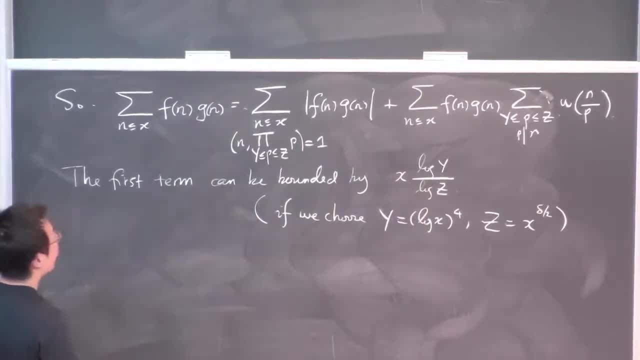 smaller than 1 over log x. OK, So the second term is going to arrange things into a bilinear estimate for me. So I'll set n over p to be the new variable m, and this becomes sum over p, sum over m, f of p, m, g of p, m, w of m. 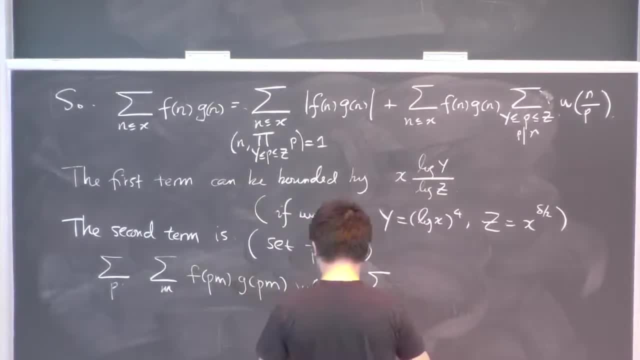 And this is bounded by sum over p. sorry, sum over m, w, m Now sum over p. there are only two ways this can go. So f of f is my multiplicative function, so f of p is can be pulled out. and then there are things. 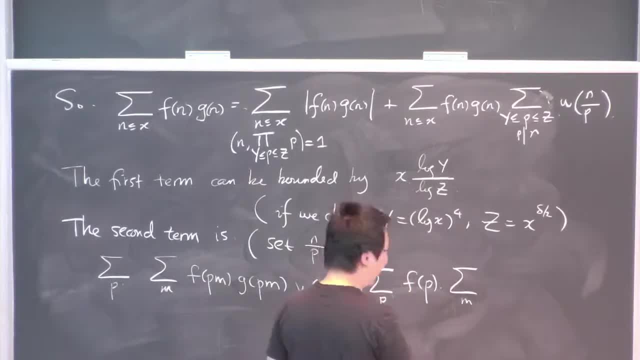 with m inside. Actually, I said there are only two ways to go, but I can go back and forth many times. Let me make sure I get it the correct. parity of times, Yeah, OK, That's what I want, and I think it's more or less correct. 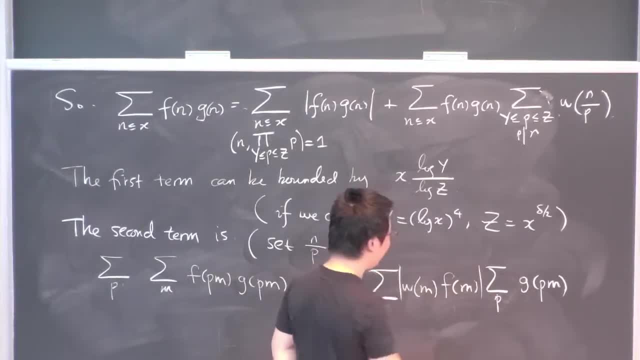 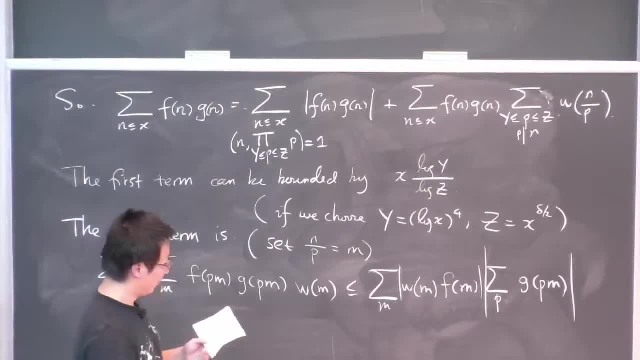 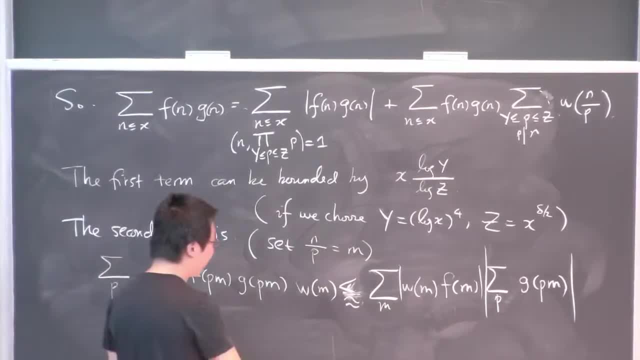 Not that I get close to it again with Cooling, and from the L2 norm of W and this quantity: Yeah, The absolute value of F is less than 1, right, Mm-hmm? Yeah, Over there, you get rid of F of P, right. 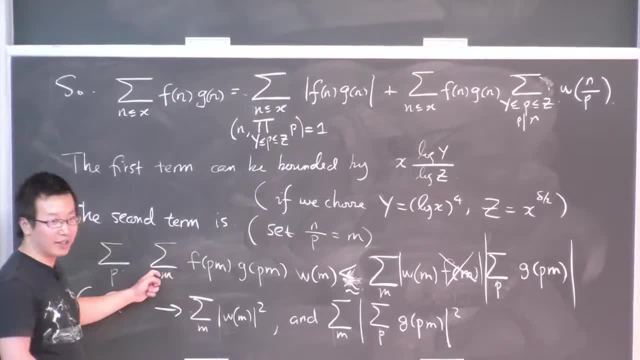 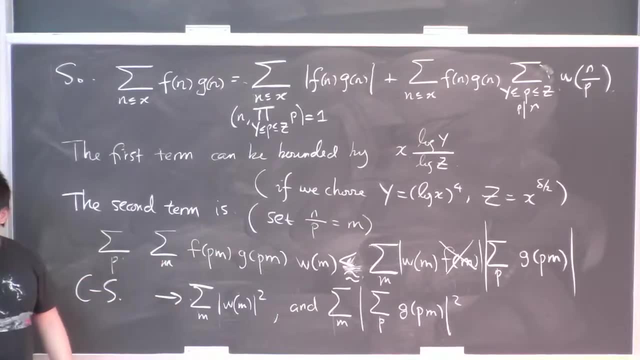 Yeah, I think I should get rid of F of P first here and then change the order of summation, But I don't think I'd- P is less than 1.. Yeah, Or just all at once, right, OK, All right. 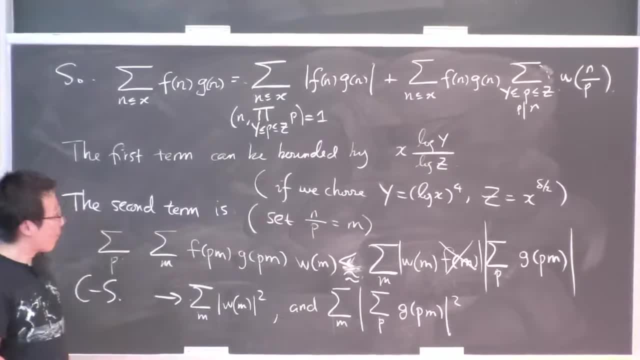 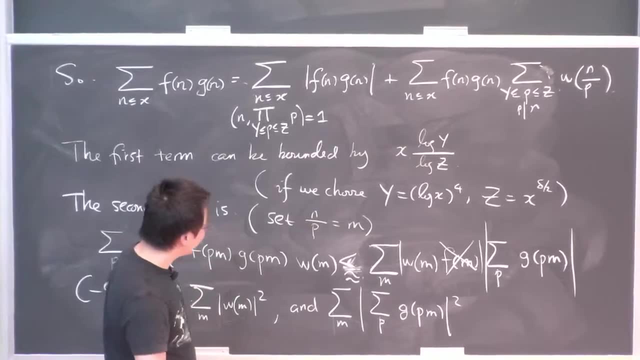 Makes sense. Yeah, Sorry, But we're just all at once if F is less than 1.. So I need to pull out this- F of P is less than 1, you just get rid of it and that's it. Yes, 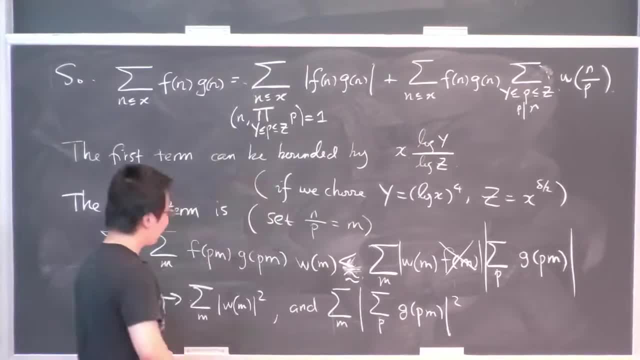 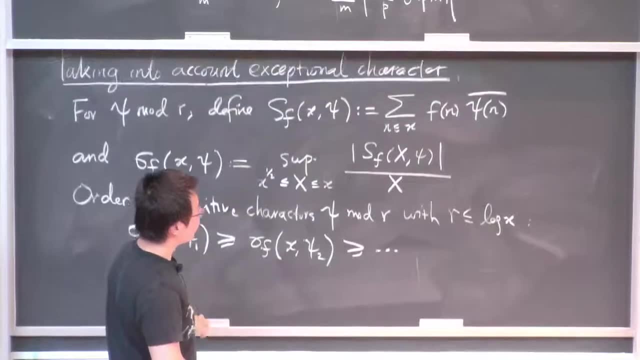 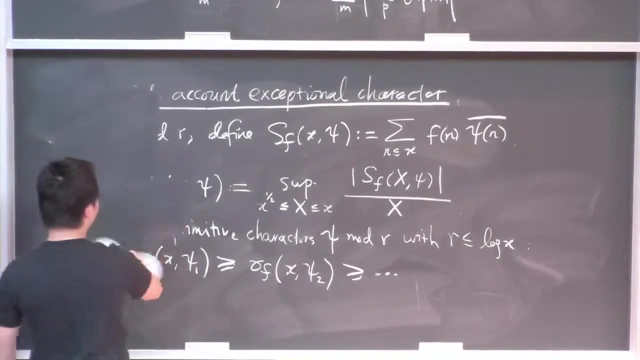 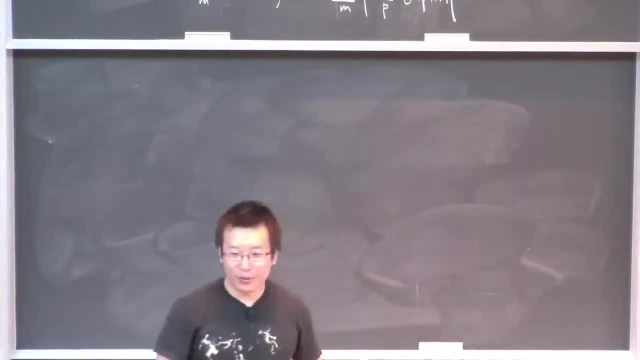 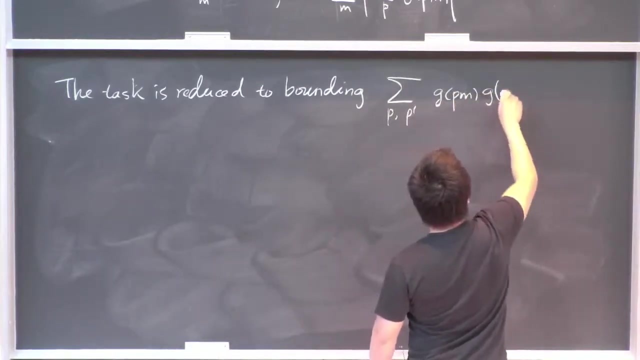 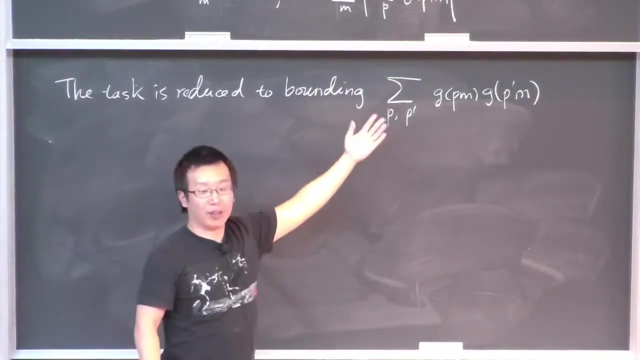 And let me just finish the approve by saying that the problem, the task, is reduced to bounding So if you expand out the square. so the point is that this is something we can understand because it only involves a function, g, which is completely explicit. 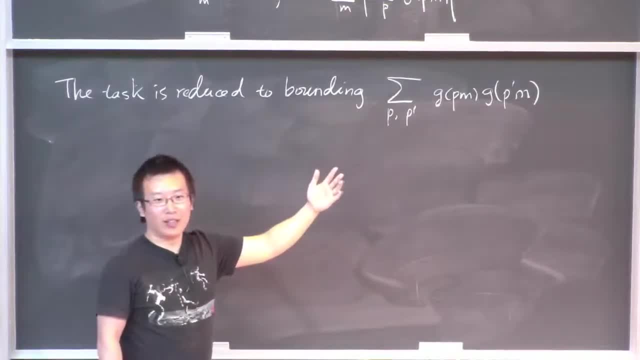 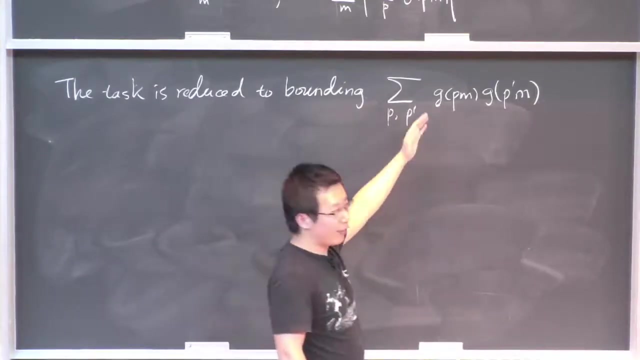 And in all of these steps we have not lost anything, at least apart from the implied constants, because the w function is something we understand, at least in terms of as far as this L2 norm is concerned. So if we can get any sort of cancellation here on average over p and p prime, then we 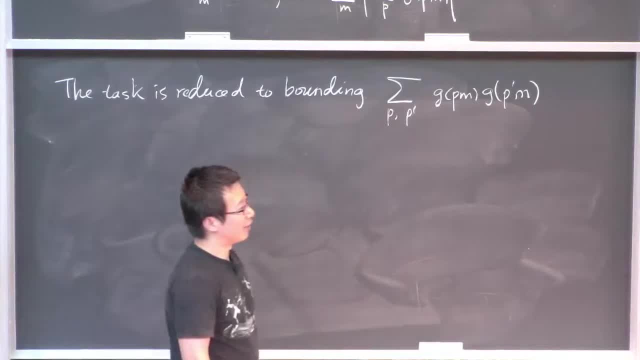 get cancellation for the original quantity And if you work it out- which is complicated but it can be done- you save roughly a w to the 1 half for this bilinear sum. Any questions apart from this last few lines? So I would like to end my talk with stating some further results, two further results. 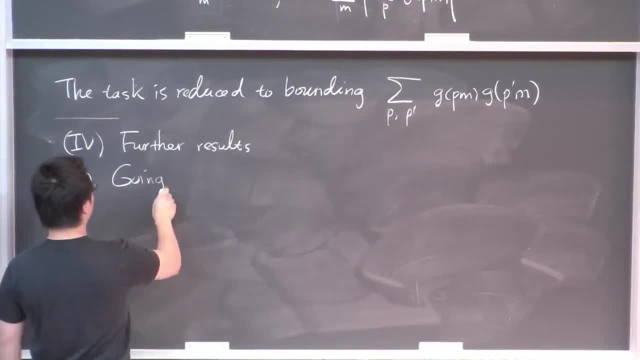 The first is about going beyond x to 1 half. Okay, So in the case of primes, there was famous work of Fouvrier and Ivaniuk that goes beyond x to 1 half, to x to 4 over 7, but at the cost that you have to use a putting the well factor. 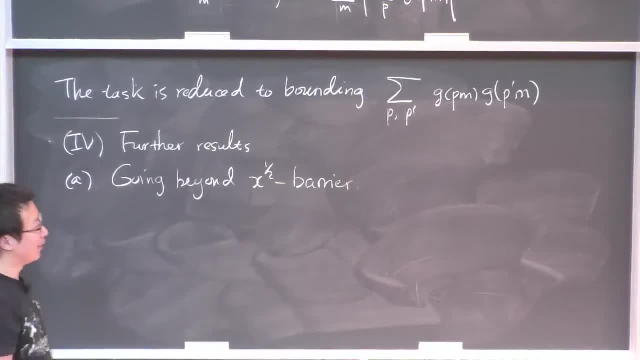 weight. or look at smooth moduli, And similarly this type of thing was done by Jan in his work of bounded gaps between primes. In the case of multiplicative functions, we can do something similar, in fact better, in a quantitative sense. 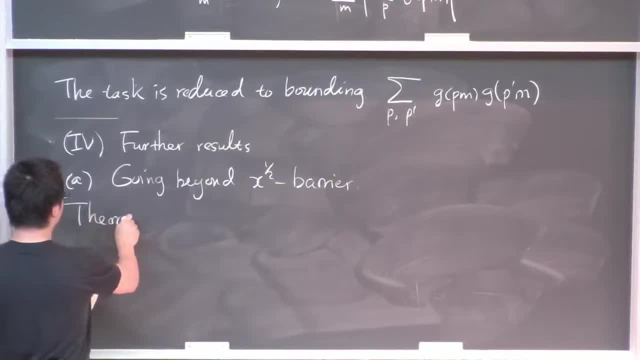 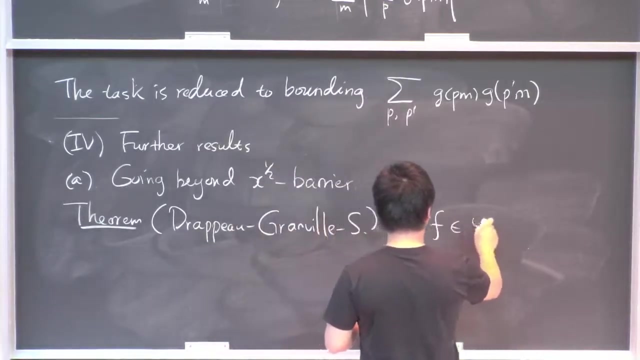 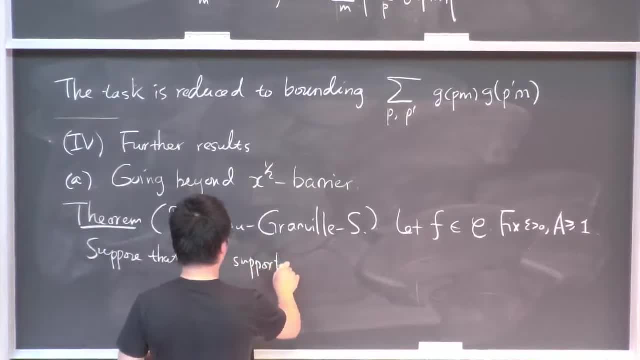 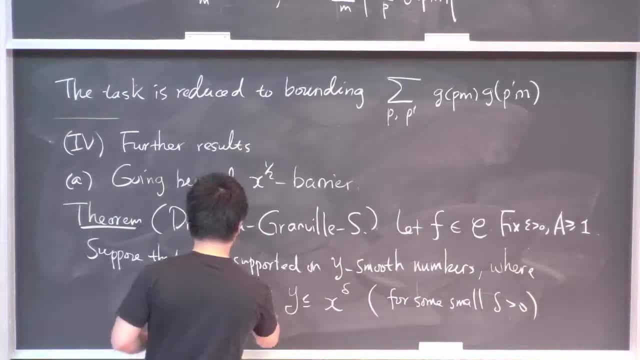 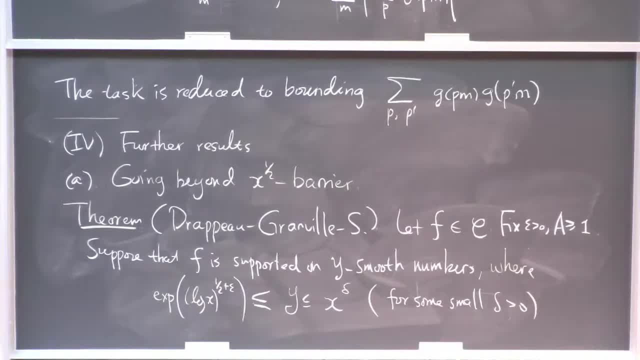 So the statement is that we have the Bon-Berge-Riven-Gradov theorem If the moduli, sorry, if the residual class A does not vary with Q and going beyond the, let's say, 2.5 to 0, this is not going to be accurate. 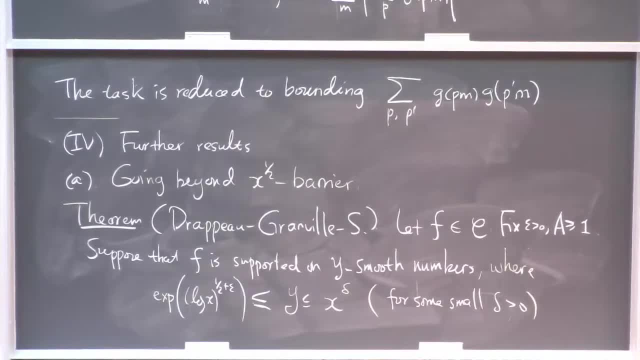 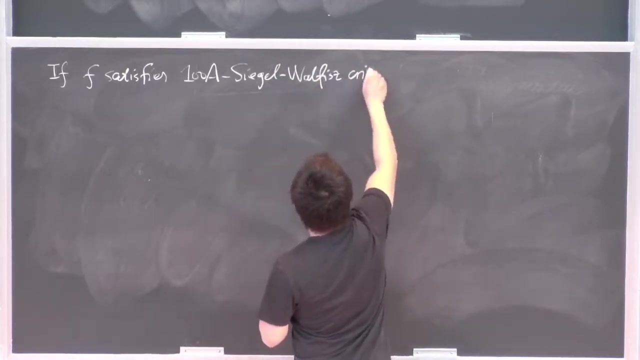 beyond the x to 1 half. So if f satisfies 100a legal warfish criterion, then some over q up to x to 3 fifths minus epsilon delta, fxq1 is bounded And you save an arbitrary power of log. where psi, xy is the number of y, smooth numbers up to x. So I don't want 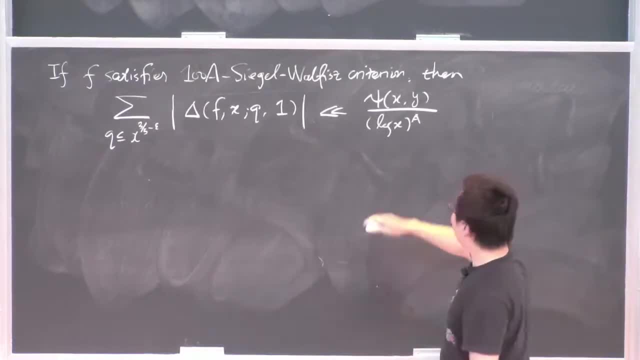 to talk too much about this, but I should just say that if you want to save log s to the power of a savings, come on Compared to the theorem before. there are large primes that could cause problems. But if I make the assumption that f is supported on y smooth numbers, then those abstractions 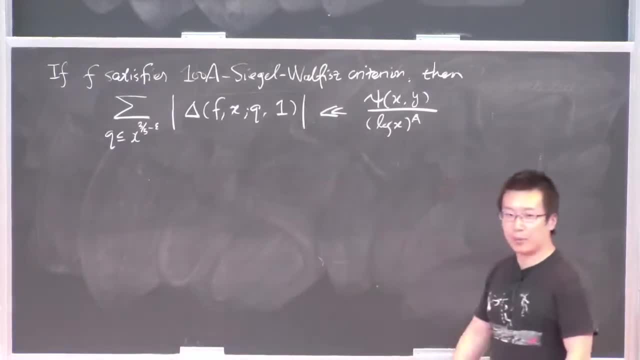 go away And I can actually expect an arbitrary power of log x saving in this context. So just to clarify: fxq1 is not Yeah, So 1 can be any fixed number, a with magnitude, bounded by a, Bounded by q, Bounded by x, to the 3 fifths. 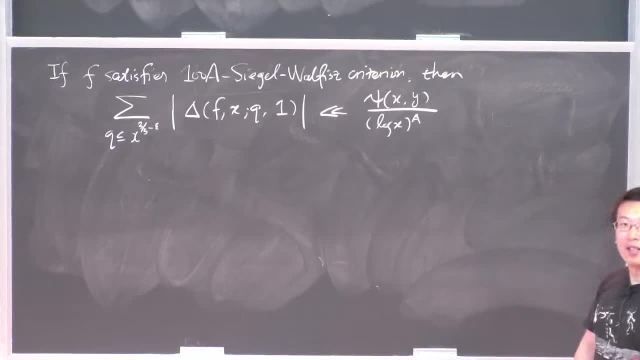 So am I allowed to replace 1 by a in my notes? Sorry, am I allowed to replace 1 by a in my notes? You can do whatever you want, but OK. So let's do this For all a. OK. 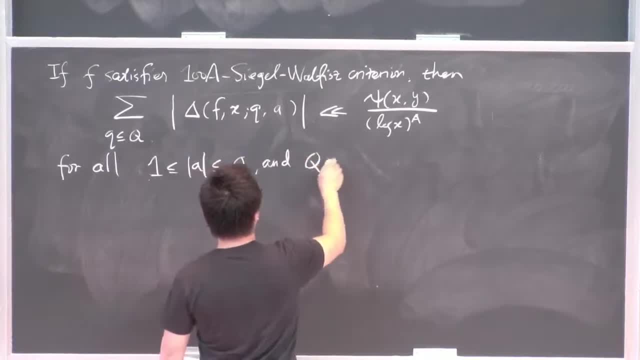 So, yeah Yeah, there is no maximum, definitely OK. so I should just say that, in the case of smooth numbers, I Sorry q and a have to be co-primed. Yeah, Yeah, Yeah, Yeah Yeah. 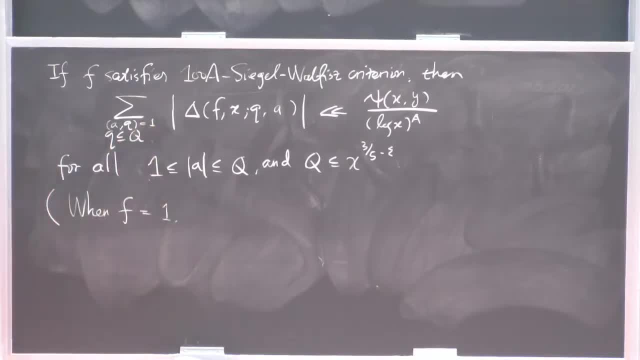 Thank you. You see, that's why I chose a equals to 1.. So in the case of the function just being the constant function, when it's now 0, so when we are just looking at y smooth numbers, this was proved by Fulvry and Tenenbaum and 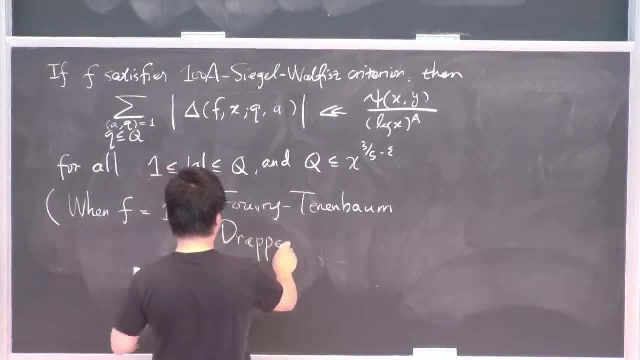 later refined by Drapeau in terms of the range of y, And in this case one can get a much wider range of y. So y can be a large power of log x, But in our theorem we were not able to do that. 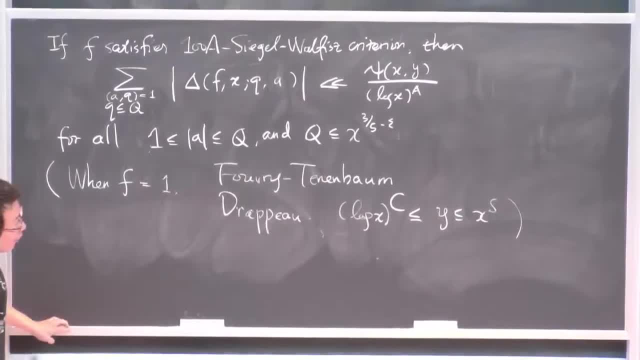 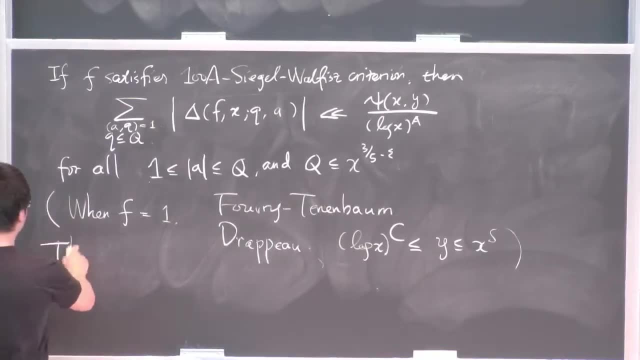 So the last theorem that I was going to mention- and I'm out of time so I'm just going to state it casually- So this is b. B is supposed to be a general theorem about when a function, an arbitrary function, satisfies Bombier-Rivine-Rogatov. 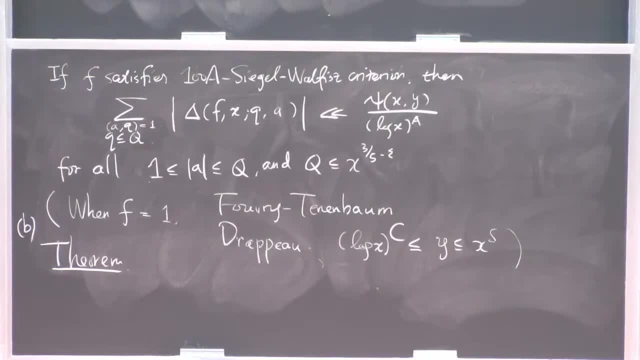 And now, when I say satisfies Bombier-Rivine-Rogatov, I mean satisfies Bombier-Rivine-Rogatov with an arbitrary power of log saving. So I think roughly, the statement is the following: that f and g be two multiplicative functions. 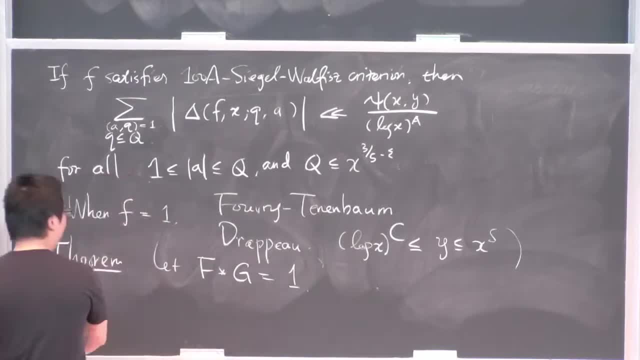 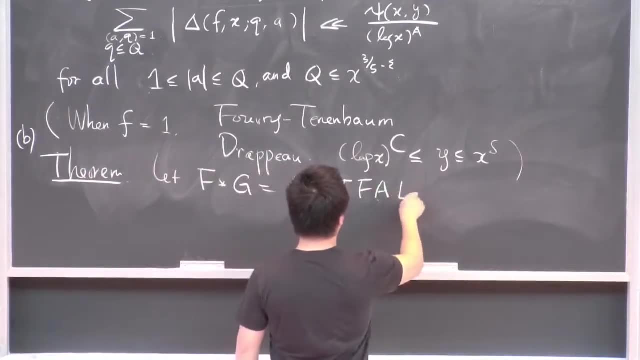 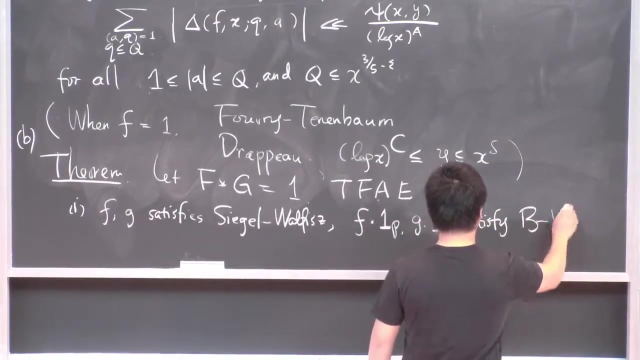 so that they are inversely inverse of each other. Then the following are equivalent: 1. f g satisfies the Eagle-Warfish, And if I look at the value value of these things at primes, so they satisfy Bompier-Rivenogladov. 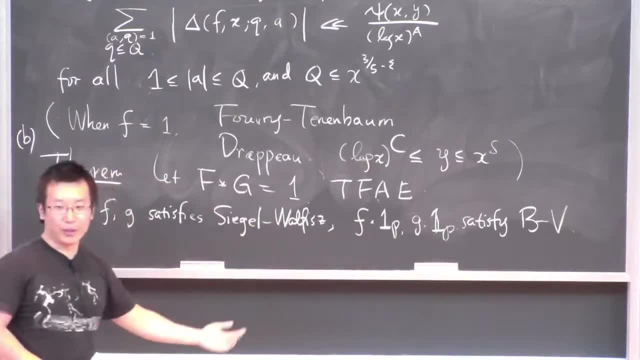 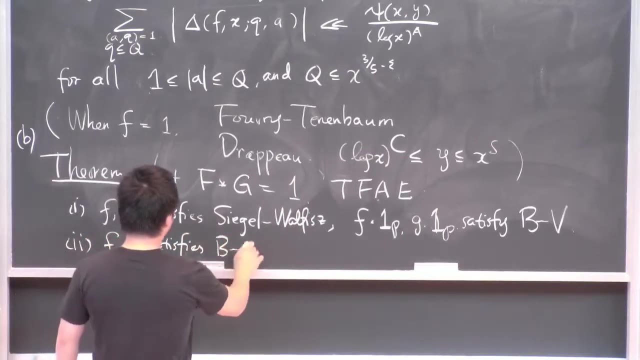 So note that when you're looking at multiplicity functions, their values at primes can be independent with each other, So you should think of this information as something given to you when you are given the multiplicity functions. And the second statement, f and g, satisfies BV. 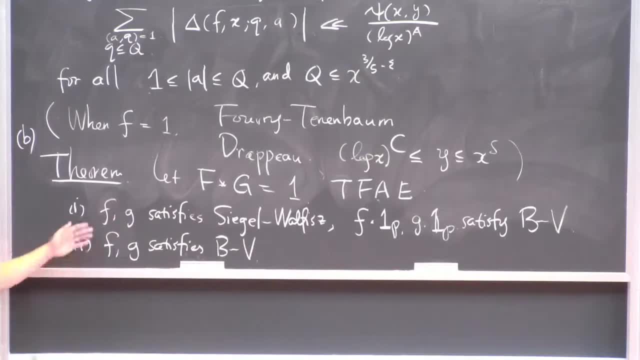 This is work in progress so I'm not going to make it precise, but some precise version of it is something that we can prove. So the interesting direction is this direction, which would imply, as special cases, that functions like mu, the Mobius function or the Louisville function, or smooth numbers, 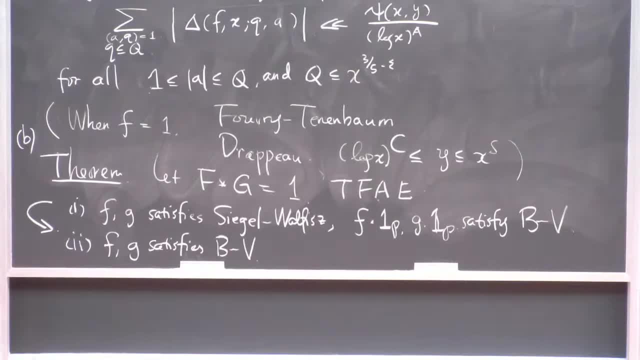 satisfies Bompier-Rivenogladov, But of course it doesn't give any new results, because the idea of the proof uses all of these previous ideas. So I'll stop here. Thanks very much, Fernando. Any questions? Yeah, 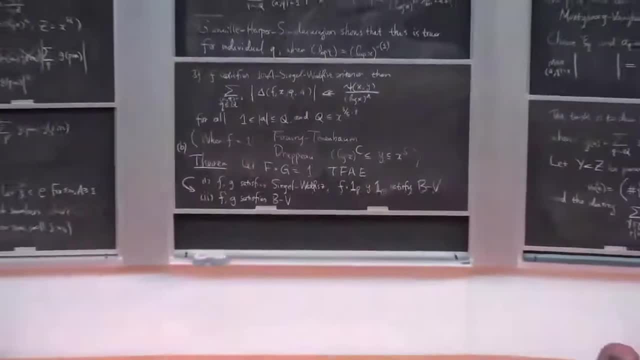 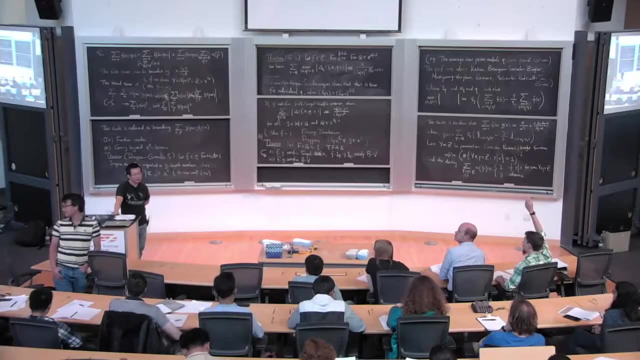 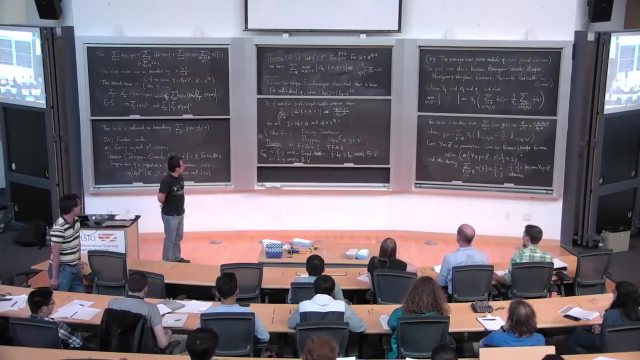 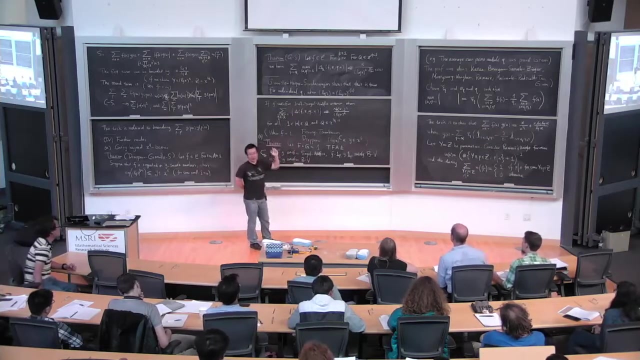 So in this final theorem you mean, I guess, one Siegel voltage, Yes, So, yeah. so let's just say that in this theorem, when I say satisfy something, I mean the inequality is satisfied for any fixed a. Yeah. 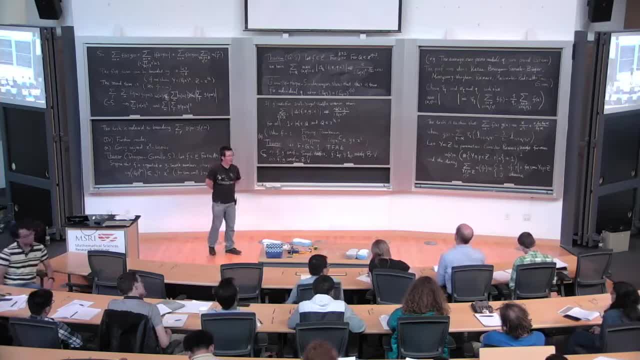 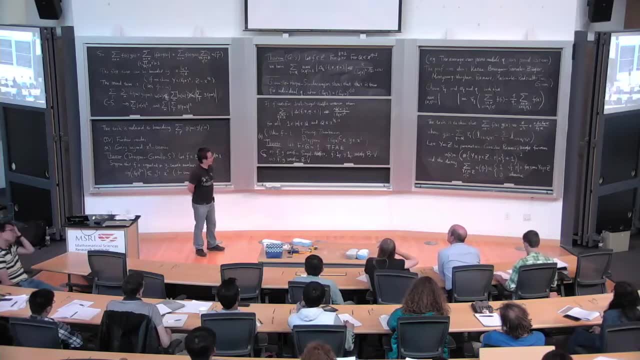 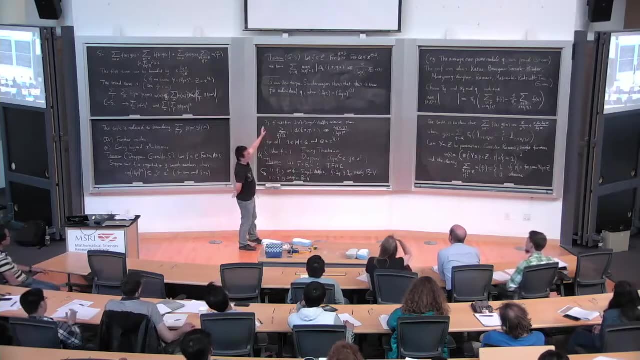 So your restriction that the values of the multiplicative function be bounded by one, Yeah, Is there any prospect of listening that? So that's a good question. So in this work of Granville sound- and sorry, Granville-Harper, and sound when you're looking- 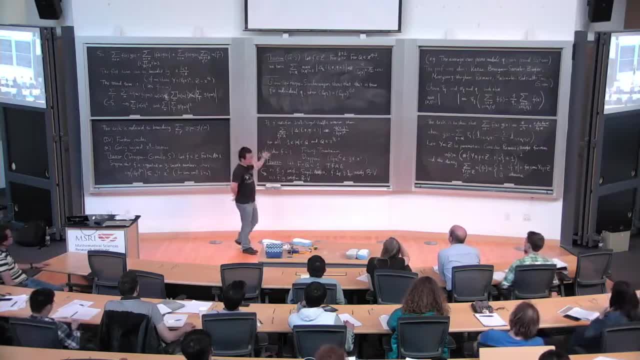 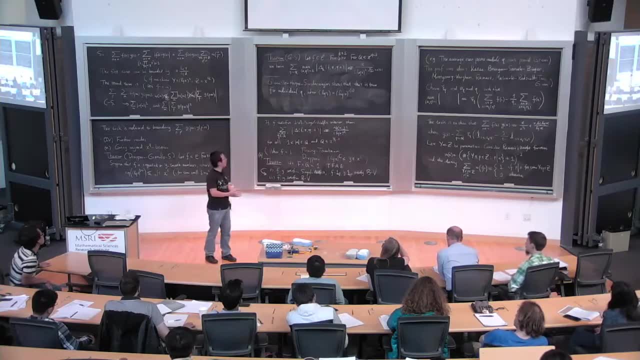 at each individual function, you're going to find that the values of each function are different. So if you're looking at each individual small module like Q, they are able to get results much more general than one bounded multiplicative functions. So they can. their result can be applied to functions, for example, functions bounded. 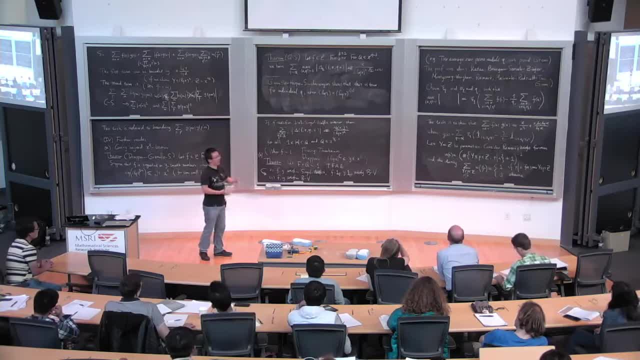 by the divisor function, But of course you expect a different bound in that case, but their results give that. However, in our BV type results- for example, this proposition that I raised- we were not able to do that, Roger. 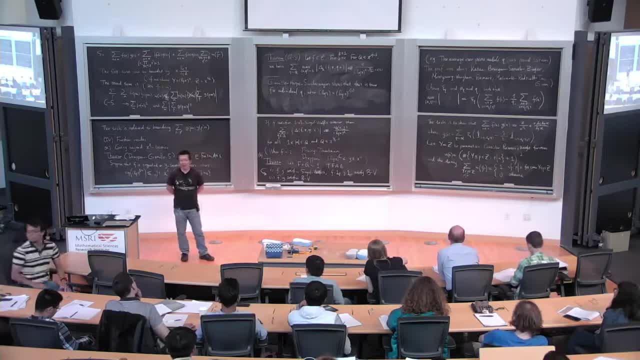 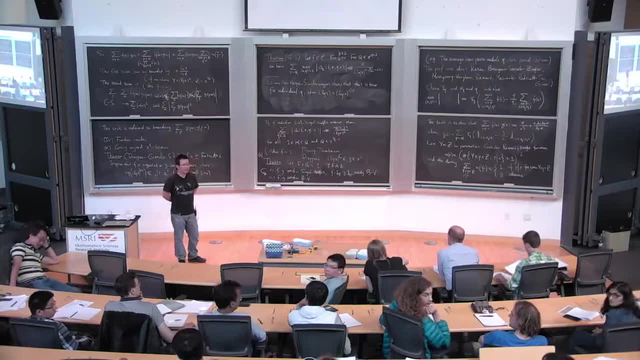 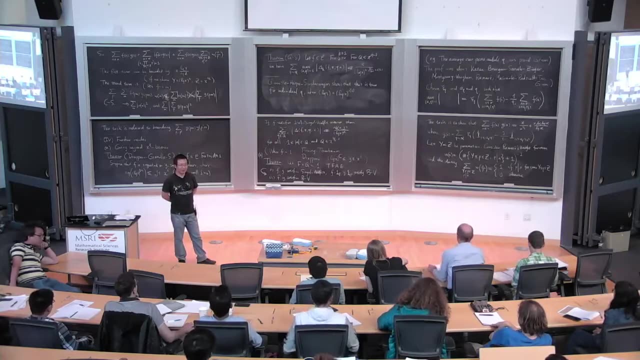 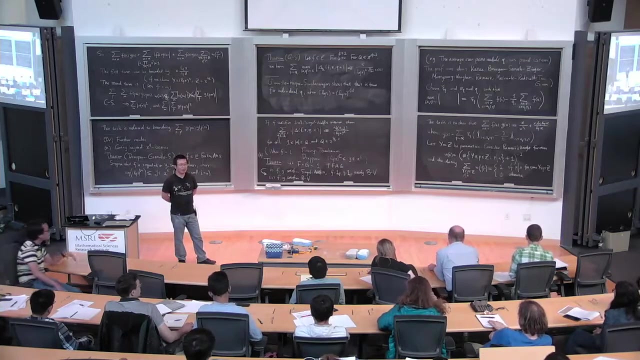 In your discussion of why you could say the first power logger, you had this set, which was a set of primes, at least one factor in the range little Q. Is it clear that the function you get there satisfies the function of the fixed a? 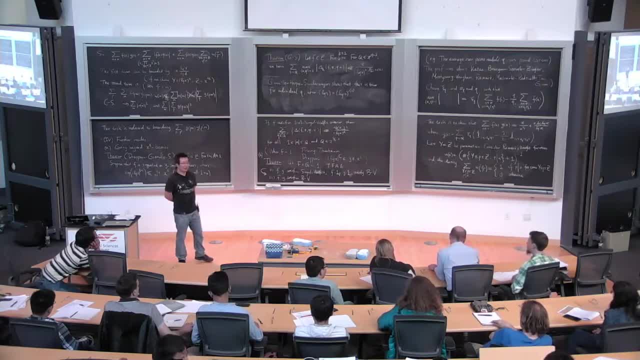 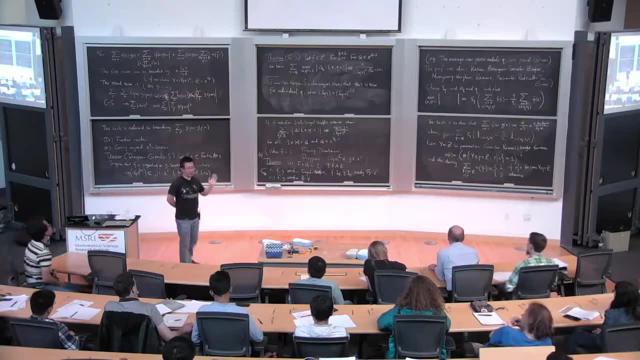 Yeah, if they're satisfied with the single log area. That's an excellent question. it's not clear. So you certainly. I think it's certainly expected that it satisfies, because there is no reason for it not to be. But so in our paper we actually prove. 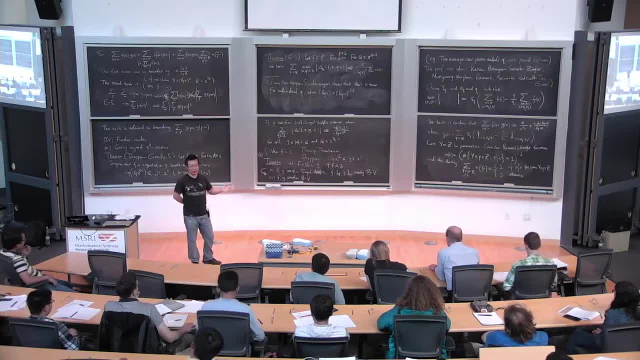 a more rigorous result with a more rigorous construction, So that construction I gave you can be modified so that you get a more well-controlled function that we can actually prove that it satisfies the single log fish And also you don't save more than log x. 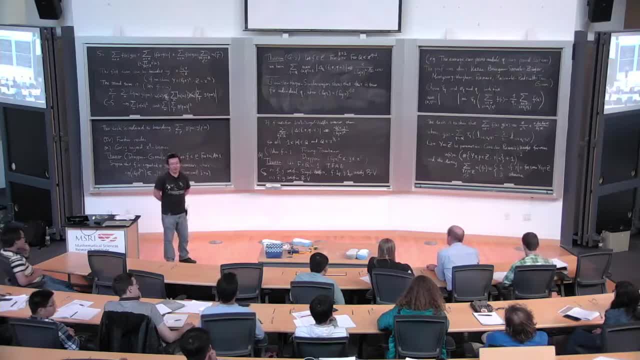 But yeah, that's a very good point. So is it expected that that set should satisfy the single log fish there? But here it seems surprising to me. I would have thought that if you insist that there is a divisor q of p minus one, 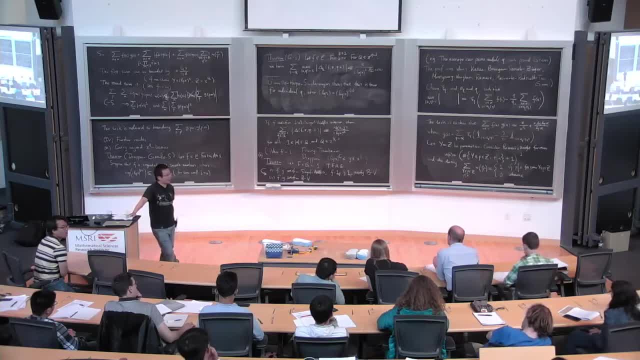 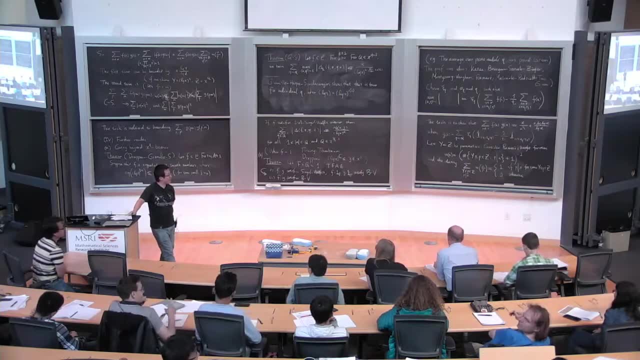 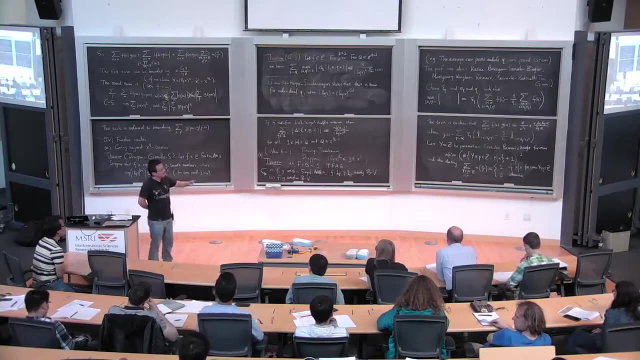 then p tends to be one mod two. Yeah, so now that you've questioned my assertion, I have doubts about it as well. but Yeah, so maybe the answer is no, but it was not a statement of any theorem, so I think I can. my comment was still valid. 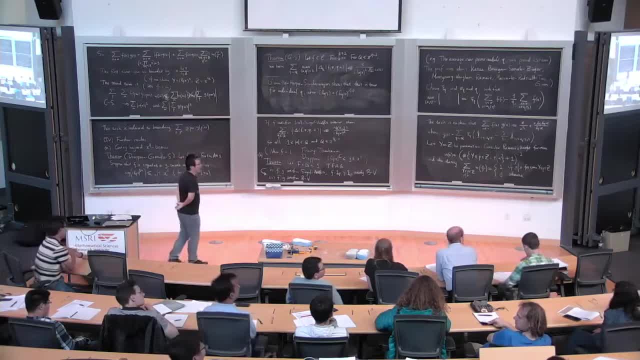 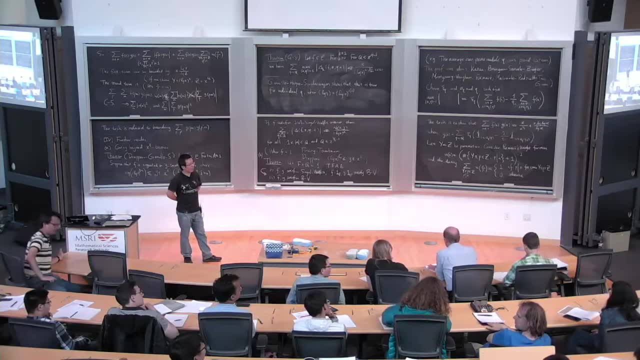 But thank you, Yeah, Yes, I have two distinct questions. The first one is related to Rogers, namely say that is there any sort of sensible condition that one might impose so as to be sure that one can gain a large power of law? 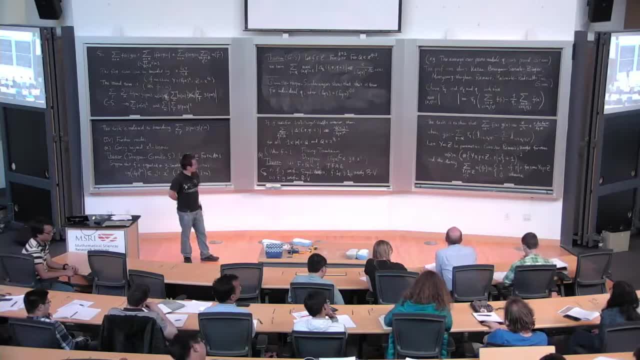 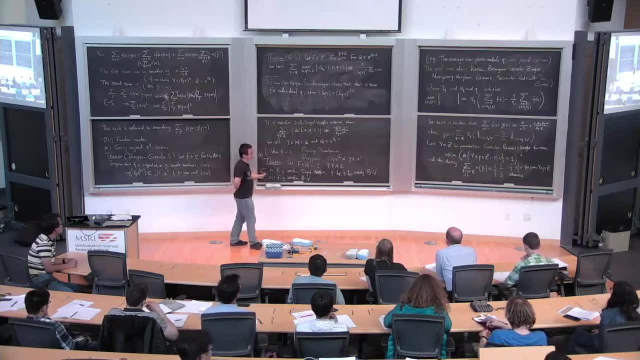 or at least so as to destroy the contrary example. Yeah, so I think this. maybe, if I understand your question correctly, this is the theorem that tries to understand that question. Yeah, but just Can you see, Just to take care of my second question, namely: 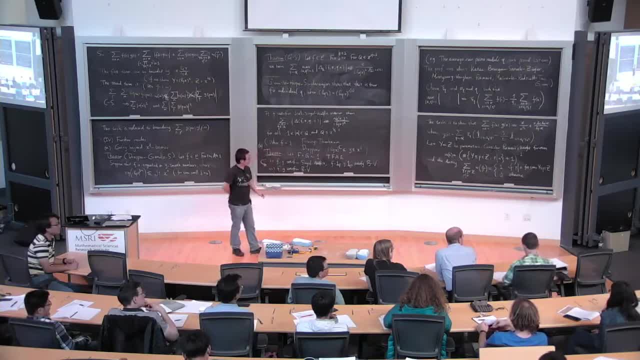 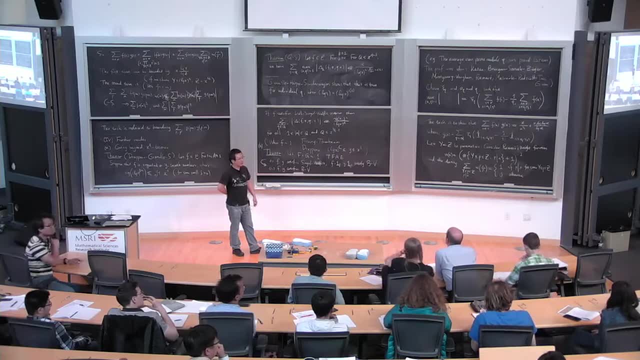 Okay, then can you repeat your first question? Well, my first question was: well, my first question was simply: what sort of condition could one impose on the functions So one might be able to hope to gain the power of law? 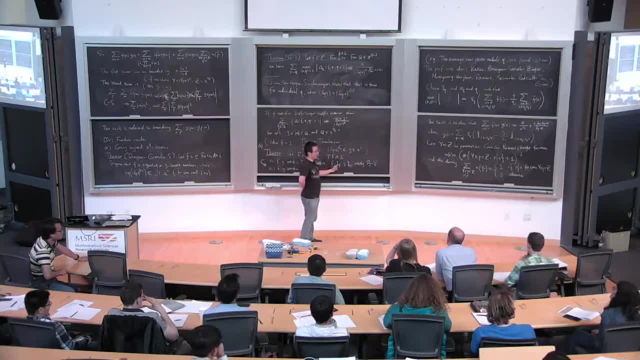 So you can hope to assume that the function f and also associate g at prime values satisfies BV with large power of log. That would imply, I see, so that's a time. So well then, I we saw my comment, the point which this: